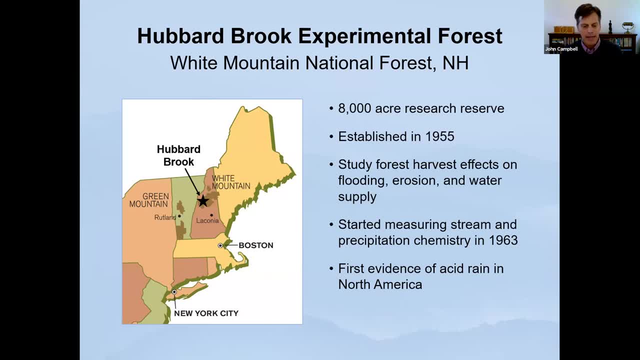 It sounds like many of you are familiar with Hubbard Brook and have heard about it. I know some of you have been there too. It's a pretty neat place. If you ever get an opportunity to visit- please don't come now, but at some point in the future. if you're interested, we'll greet you there with open arms. 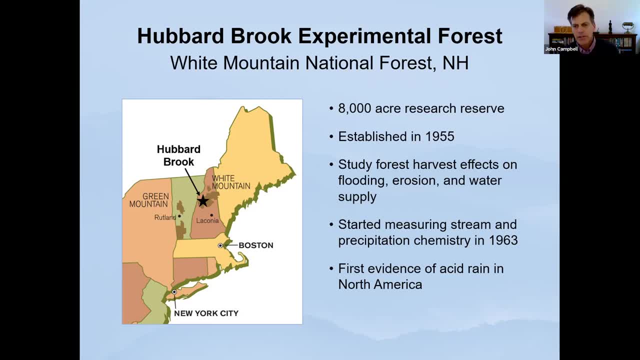 The Experimental Forest is a 8000 acre research reserve in the White Mountain National Forest. It was established as a center for hydrologic research in the northeast in 1955. And at that time there was a lot of concern about forest harvesting and impacts on flooding, erosion and water supply. 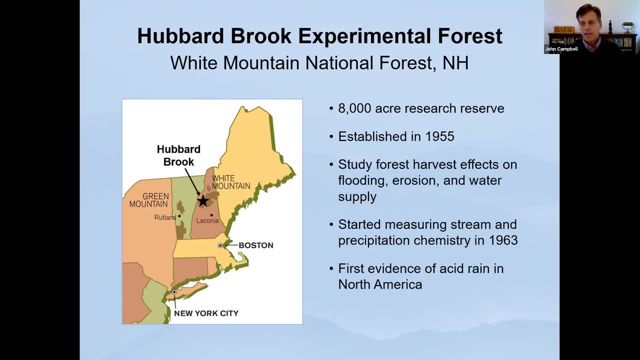 And so a lot of the early work at Hubbard Brook focused on that. Since that time the research program has really expanded and there's people from all over doing all sorts of ecological research at the site. One of the things that really put Hubbard Brook on the map is that. 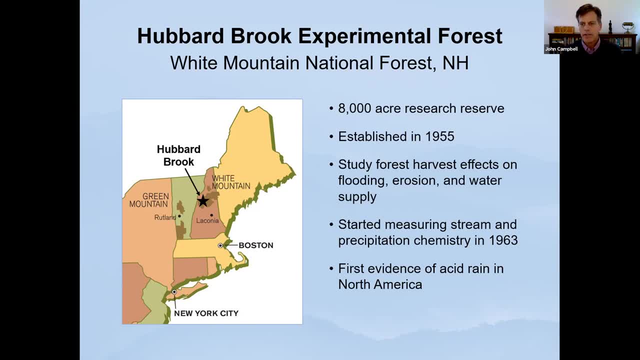 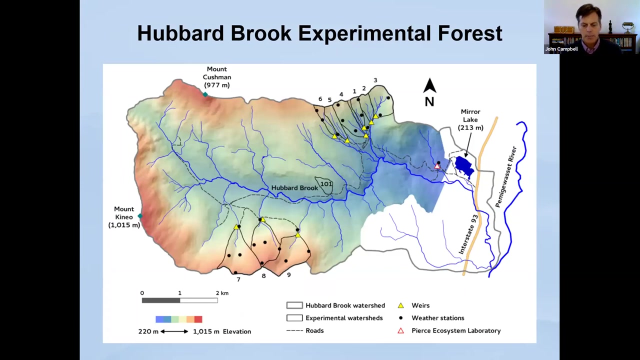 it's got one of the oldest and longest records of precipitation and stream water chemistry anywhere in the world really, And that record provided some of the first evidence of acid rain in North America and also a lot of insight on nutrient cycling in general. The Experimental Forest is six miles long by three miles wide. It's named after Hubbard Brook, which is the main drainage in the Experimental Forest. 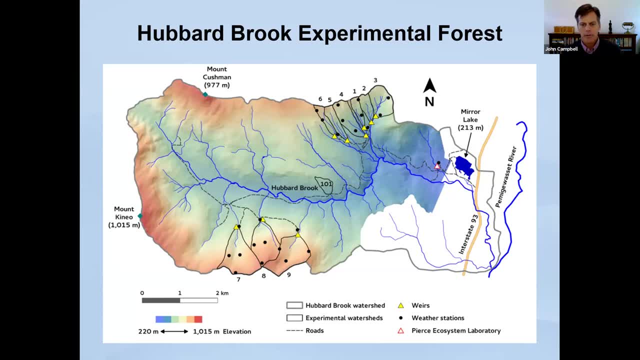 It runs through the middle of it here and the boundary of the Experimental Forest follows the boundary of that main branch of Hubbard Brook. There are a number of small gauged watersheds within that larger Hubbard Brook valley And some of these have been subjected to experimental manipulations, primarily cutting experiments. but also a calcium, a whole watershed, calcium addition. 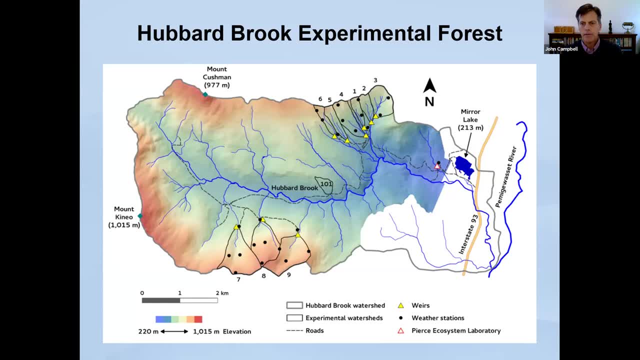 There are a number of places where we monitor climate, So we have a network of weather stations, And there are other things being monitored at the site, like soil, vegetation and animals. The major research theme at Hubbard Brook is ecosystem response to disturbances, And so this includes things like forest harvesting, air pollution. 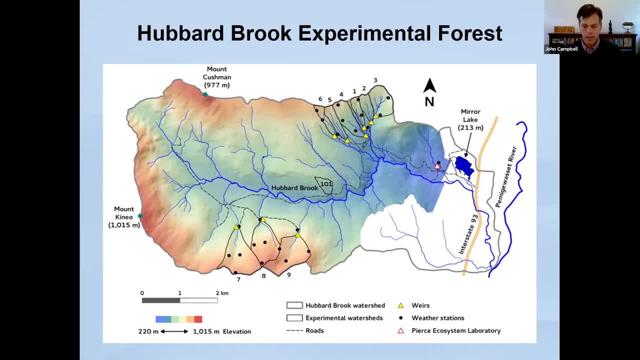 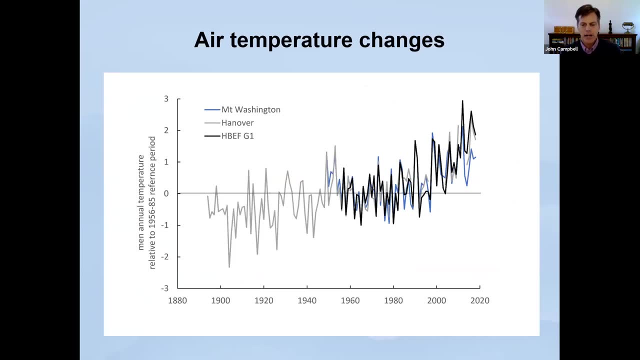 and, of course, today's topic, which is climate change, And it's clear that the climate is changing at this site and really in this region. These are air temperature data from Mount Washington, Hanover, New Hampshire and the Hubbard Brook Experimental Forest. 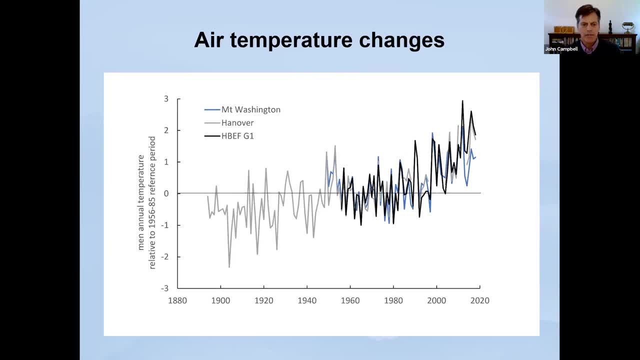 This is expressed as an air temperature anomaly, So it's a deviation from the mean in degrees Celsius And we present it this way so you can compare these sites with very different temperatures on the same scale. And you can see that at Hubbard Brook the air temperature has increased Since the 1950s. it's increased by about one and a half degrees Celsius over the 60 plus year timeframe. 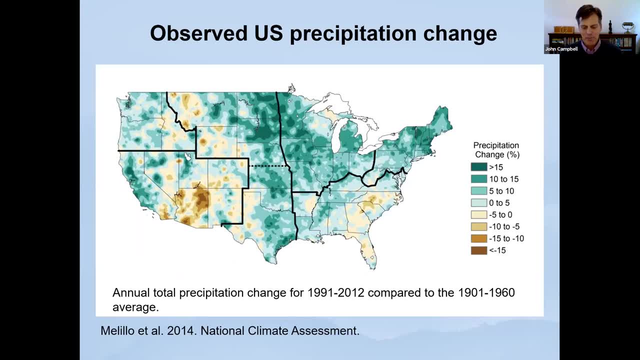 When people talk about climate change, they often think more about air temperature and less about precipitation, but certainly precipitation is changing as well. This map is from the National Climate Assessment and it shows precipitation change from the first part of the century to the latter time period. 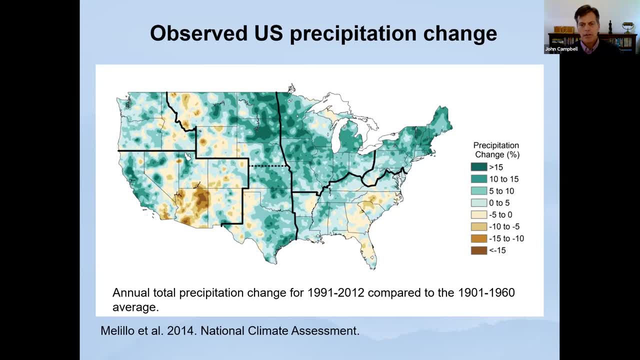 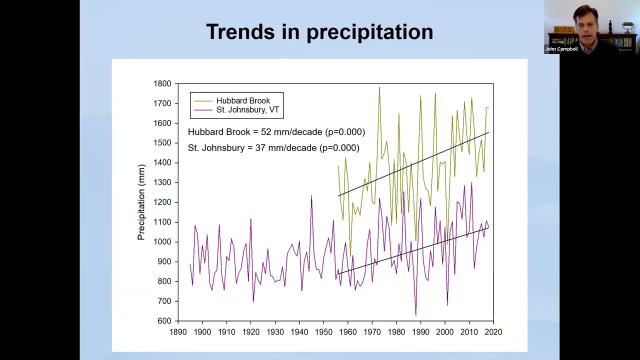 And you can see that there's really been an increase in precipitation in the northeastern US anywhere from you know five up to greater than 15% increase, And so we have seen these increases in precipitation And the record at Hubbard Brook bears that out. This is the precipitation in gold at Hubbard Brook. 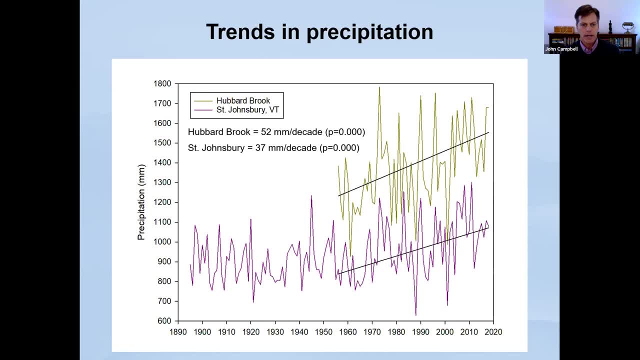 And the purple here is from St Johnsbury, Vermont, which again has a record that dates back to the late 1800s. You can see the precipitation kind of bounced along, you know, from the late 1800s up until about the middle of the 20th century. 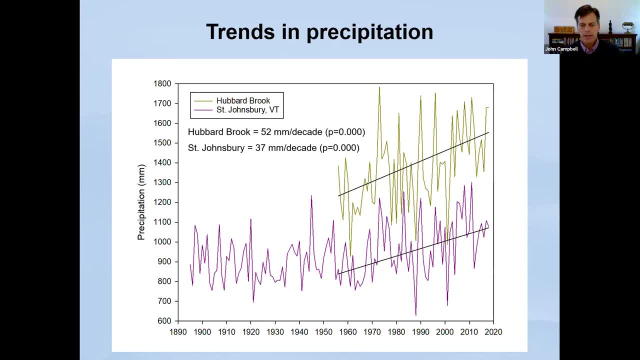 And then we've really been on this sharp increase since that time. At Hubbard Brook, you know, right around when the record first started, the precipitation just kind of took off, And so, although there's a lot of variability from year to year, this increase is really quite dramatic. 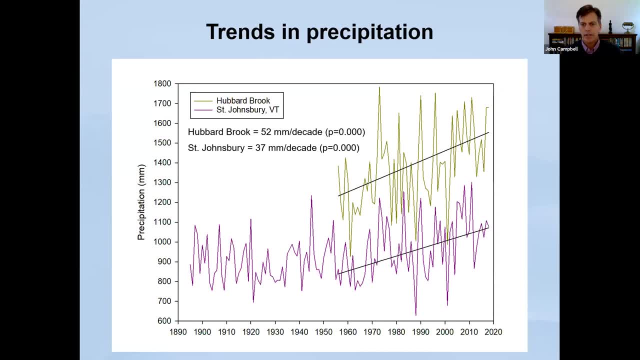 It's about a foot increase over this 60 plus year record, And so you know that's just really amazing when you think about it. I'm not convinced we can attribute that all to climate change, but clearly we are in a very wet cycle right now. 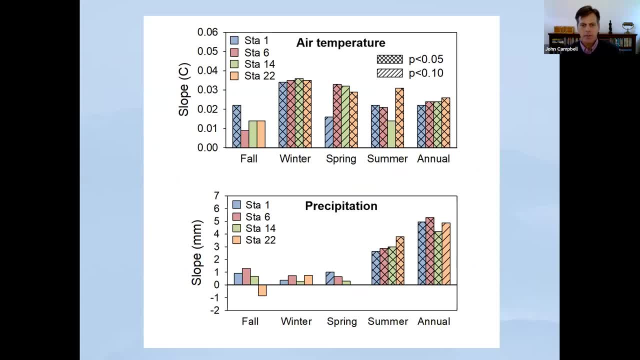 We can also look at seasonal trends in air temperature and precipitation. These are from four weather stations at Hubbard Brook And this is the slope of the trend line. So positive values indicate an increasing trend, negative values indicate a decreasing trend, And here the hatch marks just show the level of significance of the trend. 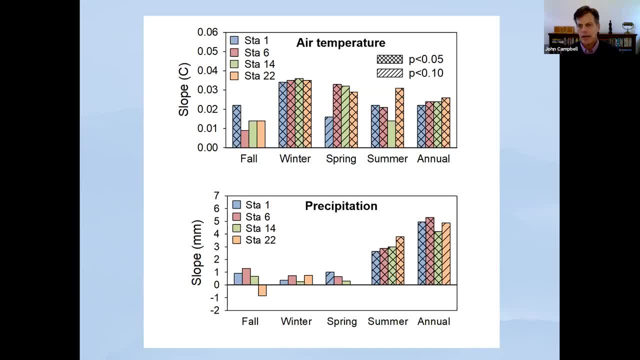 And so in the top graph if you look at air temperature, you can see we have pretty consistent increases across all seasons and highly significant increases in air temperature on an annual basis. For precipitation we see very little change in fall, winter and spring maybe slight increases, but not much of a change. 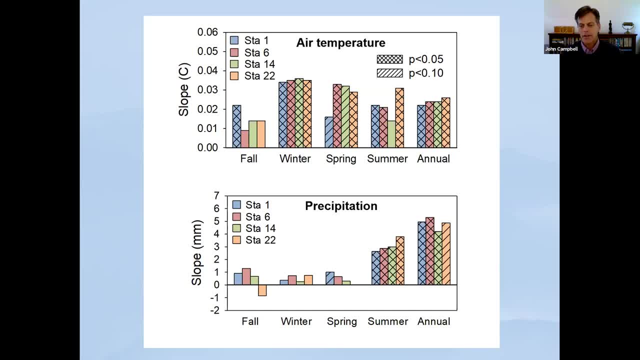 Really, the bulk of our precipitation increase has occurred during the summer months, And this is actually, you know, the opposite of what most climate change projections are suggesting for the future. Most projections suggest we'll see more winter precipitation and little to no change in summer precipitation. 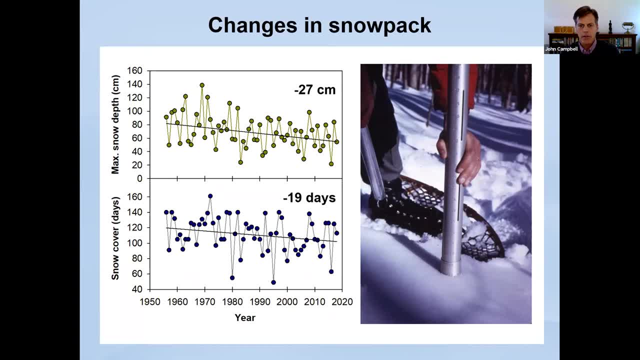 So I said we had warmer winter air temperatures and no change in winter precipitation, So it's not surprising that our snowpack is declining Again. this is really across the region and there's a lot of evidence for that. At Hubbard Brook we've measured the snowpack the same way really since the inception of the study in the mid 1950s. 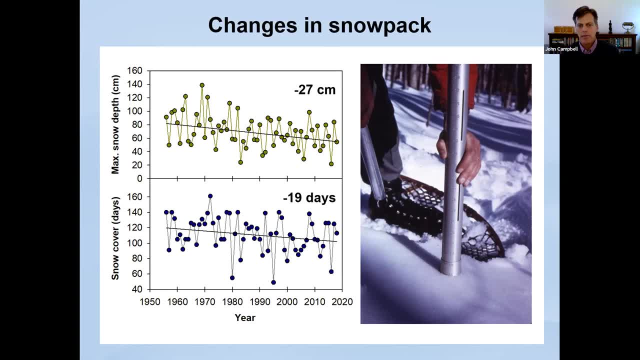 The top graph here just shows the maximum snow depth on an annual basis, and it's declined by about 20 centimeters, So again by nearly a foot, And the number of days of snow cover have also declined. We have about 19 fewer days of snow cover now as compared to when. 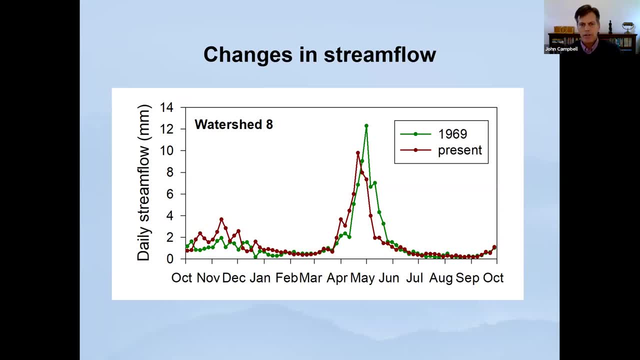 that record first began. The changes in snowpack have also led to changes in streamflow. These are streamflow measurements from one of our reference watersheds, so it's relatively undisturbed, And here I'm just showing streamflow for the present compared to or at the end of the record compared to the beginning of the record. 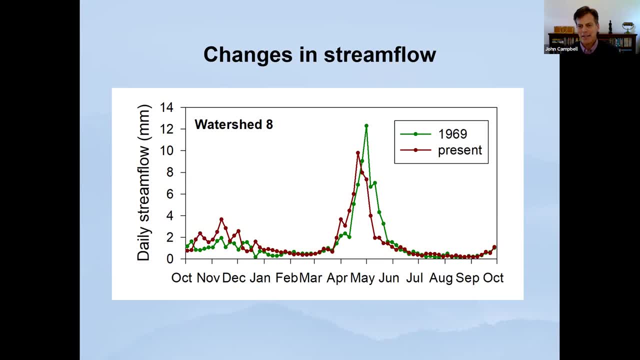 And so it's not actually the year 1969.. It's the beginning of the trend line and which started in 1969 for this watershed, And so you know, the overall pattern of streamflow at Hubbard Brook and in most of these streams in the region is that. 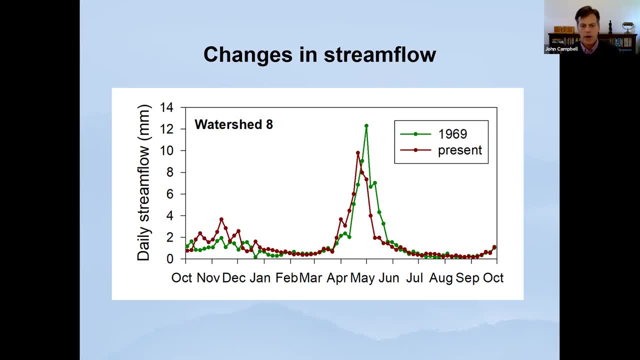 you tend to have higher flows during the fall and into early winter. Then we have low snows, as that precipitation accumulates in the snowpack and then it's released over a very short snowmelt period in spring And then we have again low base flows, And so in summertime when there's a lot of transpiration. 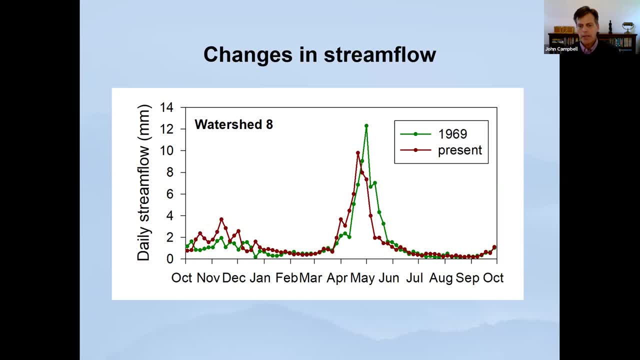 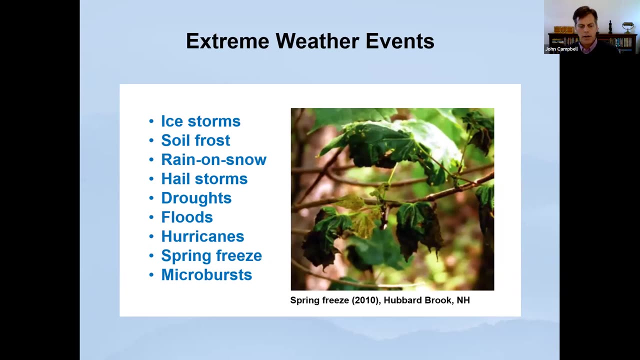 And so we're seeing this shift. The snowmelt peak isn't as high as it used to be, And it's also occurring earlier in the year, And we tend to have higher flows as well in the early winter months. Okay, so far I've talked almost entirely about long term trends. 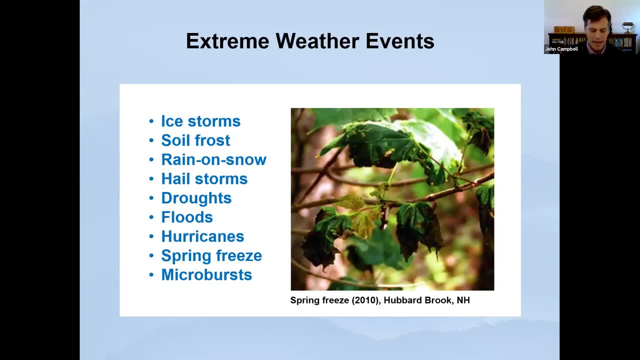 And I just want to make the point that extremes are. these extreme weather events are also important and can be even more important than these more subtle changes that occur over time. We have lots of evidence of these extreme events, the occurrence of the events and how they've impacted. 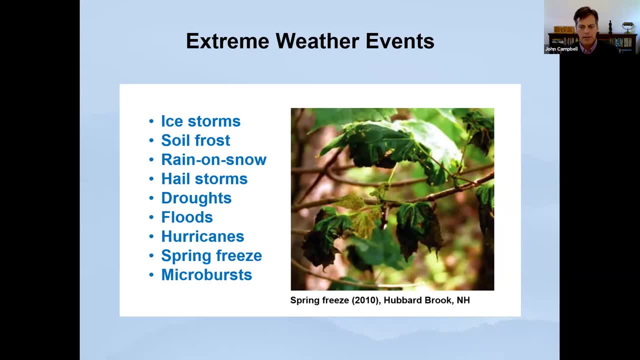 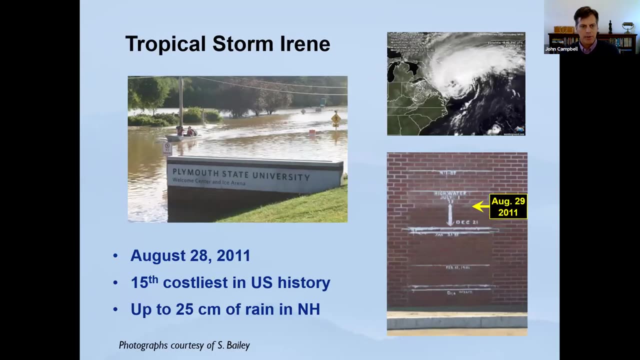 the hydrology and biogeochemistry of these systems and nutrient cycling in general, And these are some of the more prominent kind of climate extremes or weather events that we've seen at Hubbard Brook. A good example is Tropical Storm Irene. I know many of you were affected by this in some way. It was. 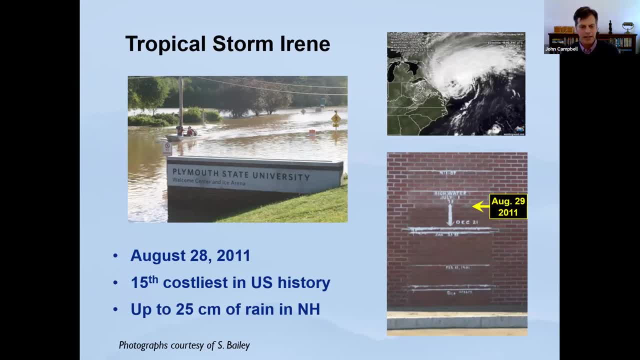 occurred in 2011.. It was the 15th costliest hurricane in US history. At the time it happened it was the seventh costliest- So clearly we've had a lot of these big hurricanes in recent years- And it dropped up to 25 centimeters of rain in New Hampshire over a relatively short period, basically over a 24 hour period. 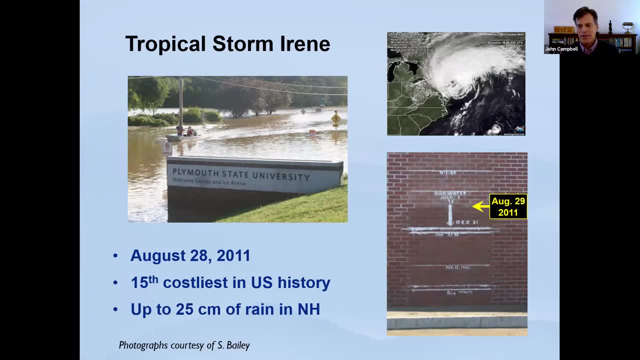 This event was not unprecedented. I love this picture in the lower right here. It's on the side of a gas station in Plymouth, New Hampshire, And it shows the high watermark for Hurricane Irene and the high watermark of other storms. And so there were at least two other storms. 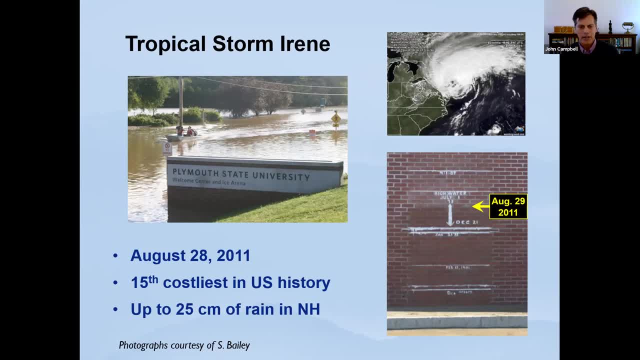 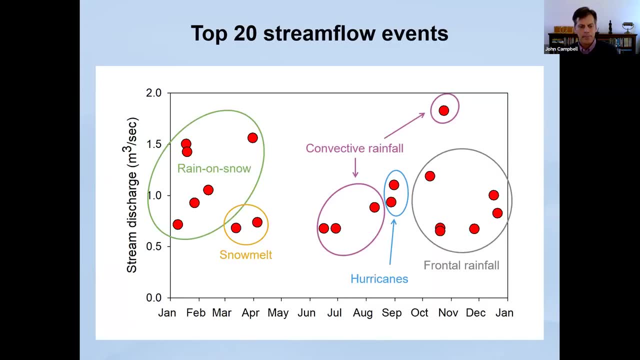 that were higher than the high water market at Hurricane Irene, And so we do get these events and they're quite damaging and costly. In one of the previous slides I showed that streamflow is highest during that snow melt period, which is true on average, but we can get flooding events anytime throughout the year. 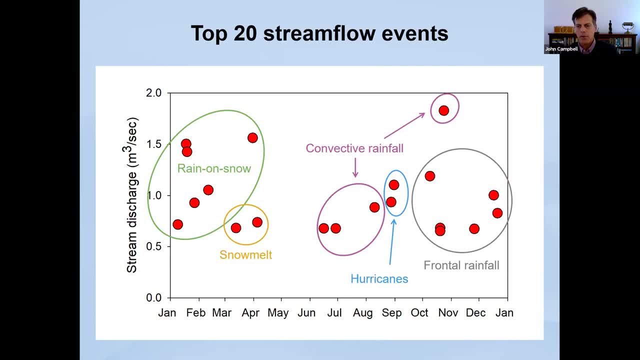 And so this is a graph showing the top 20 streamflow events at Hubbard Brook and when they occur, And we've also linked the type of event that caused these high streamflows. And so you know, you can see, that in the winter months we have rain on snow, events that can be quite important. 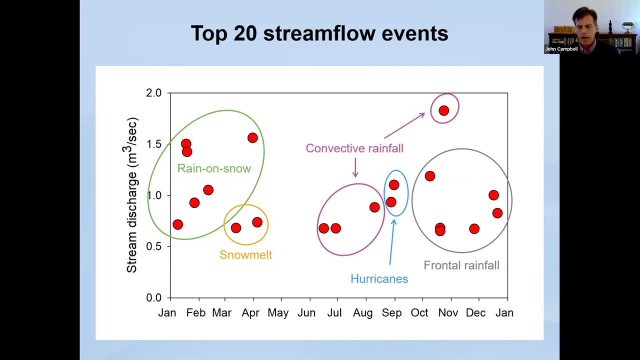 Straight snow melt events in the springtime. In the summer we get these convective rainfall events that often cause flooding, In some cases hurricanes like Hurricane Irene is one of these points here- And then in the fall and winter we have these frontal rainstorms where warm air meets cold air. So any of these can can cause flooding throughout the year. 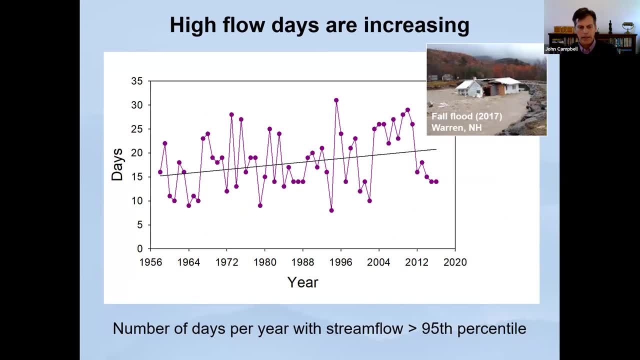 We can analyze the occurrence of the high flow events to look at how they've changed over time. Again, these are data from Hubbard Brook and this shows a number of days when streamflow exceeds the 95th percentile, And so we're seeing an increase in the number of days with high flow. 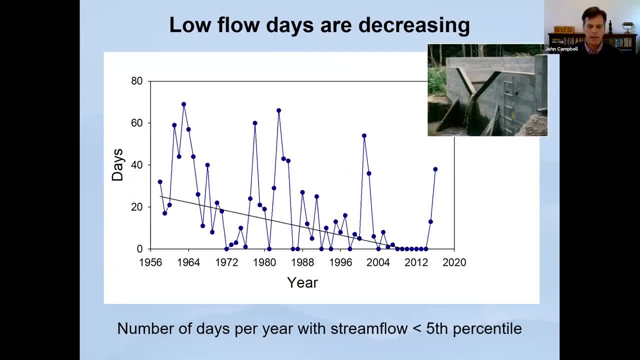 We can do the same kind of analysis with low flow. This is the number of days per year with streamflow less than the fifth percentile, And so the number of low flow days are decreasing. We often, you know, associate a drought with climate change, And so you know, so far that really has not been. 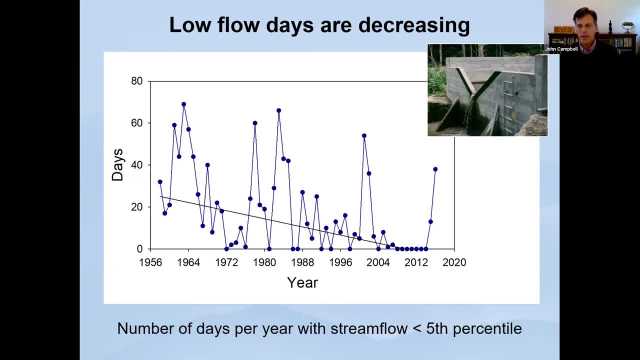 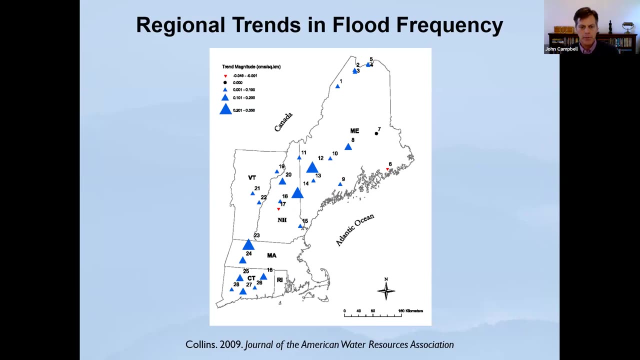 the case. We've seen an increase in base flow during summertime and that's largely because of this precipitation increase that's occurring over the summer months. The trend in flooding is really throughout the Northeast region. This map is a little dated now but it shows the trend in flood frequency throughout the Northeast. This is on major rivers. 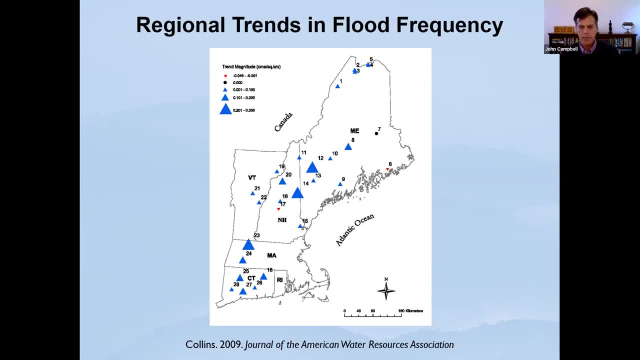 That have at least 50 years of data, and these are minimally disturbed rivers, so they're not affected much by human influences like water withdrawals and things like that, And so the blue triangles just represent an increase in flood frequency and the red triangles show decreases, And so you know most of these rivers are showing increases in the frequency of floods. 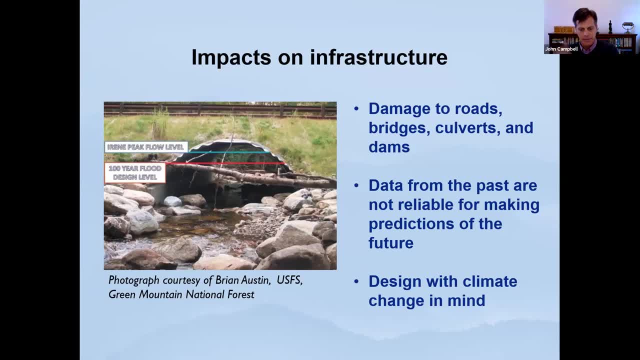 Of course, these flooding events can have massive impacts on infrastructure. This is an image from the Green Mountain National Forest. It shows the 100 year flood design level for this culvert and then it shows the peak during Hurricane Irene, And you know this particular culvert survived this storm, but many did not, And so you know. I think it just brings on the point that 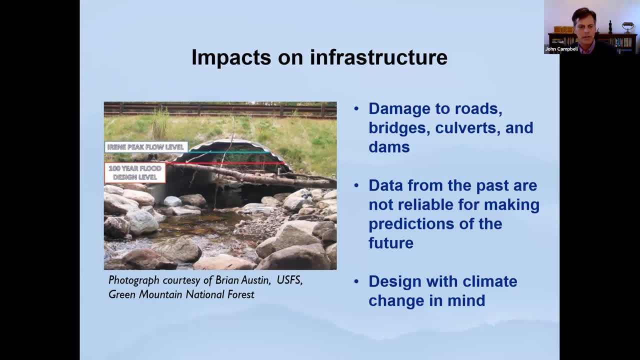 data from the past are really not reliable for making predictions for the future, And so if you have something like a culvert that you expect to last 50 years, we really have to consider how climate and precipitation might change over that long term, And so it's important to design these structures with climate change in mind. 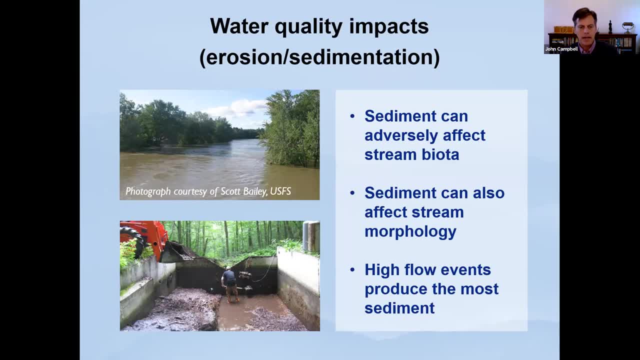 In addition to flooding events affecting, you know, infrastructure, they also can impact water quality and certainly, sediment is largely affected by these high flow events. Sediment can not only affect biota, but can also affect stream morphology and can cause these stream channels to shift. 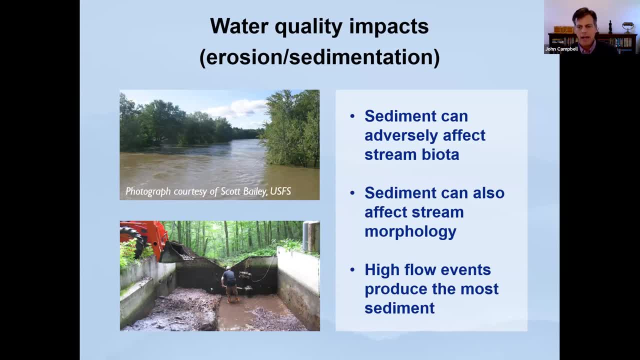 And it's really these high flow events that produce the amount of sediment. At Hubbard Brook we measure sediment in the Weir Basin, which is what this bottom image shows, and we have lots of evidence that shows that most of the sediment movement occurs during these really high stream flow events. 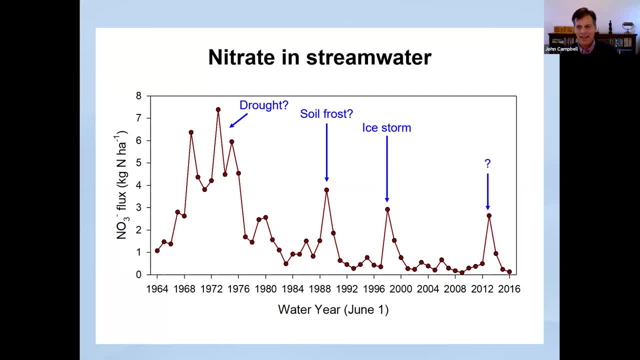 In addition to sediment, we can also talk about nutrients in stream water and how they're affected by climate. This graph shows a long term record of nitrate in stream water in the reference watershed at Hubbard Brook. Of course we're concerned about nitrogen because, although it's often a growth limiting nutrient in forest, it can also be a pollutant in stream water, And so nitrogen is very important from a biological perspective. 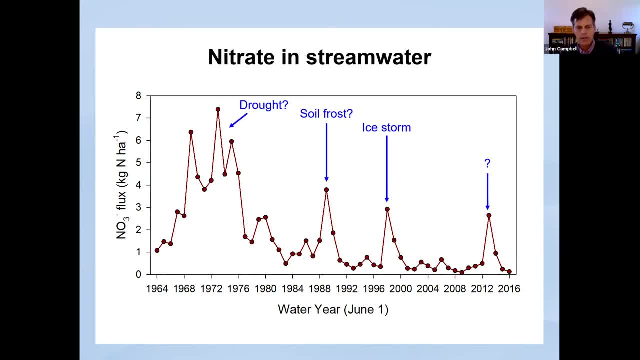 And when the watershed is disturbed in some way, it often results in the release of nitrate to stream water, And so you can see that there are a number of peaks in this long term record. I don't think we have a great handle on what's causing these peaks, but there's been a lot of speculation on what might be driving each one. 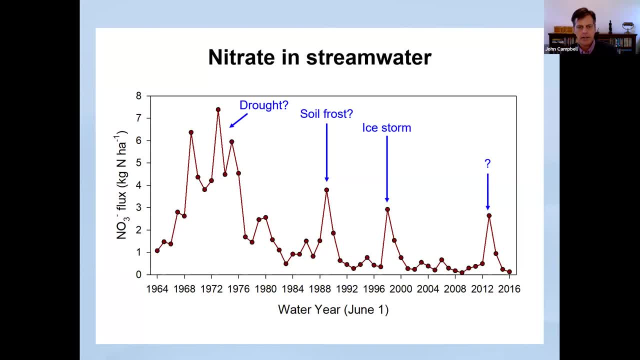 There is this period of extended high nitrate export during the late 1960s and early 1970s, and some have suggested that the prolonged drought of the 1960s that affected much of the Northeast led to this increase in nitrate in stream water. 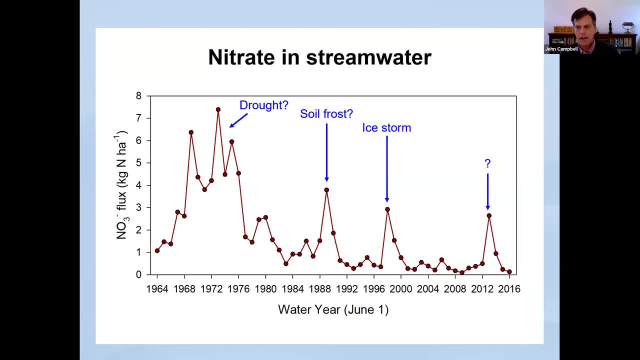 There was another peak in 1998, which we think could be due to a major soil frost event that occurred. Again, this was a regional peak in nitrate that was observed at a number of small watersheds in the Northeast. The one we are fairly confident is the ice storm of 1998.. Again, this was a major disturbance, above ground disturbance that causes spike. 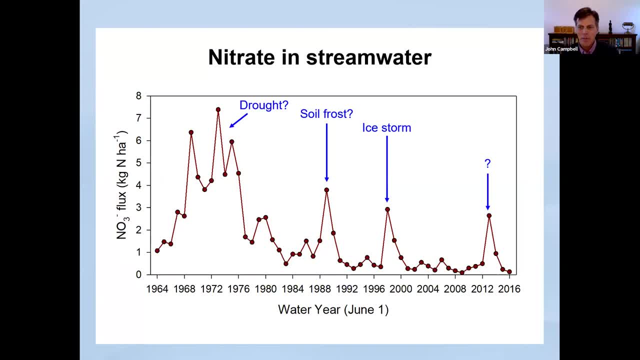 And then we had a recent spike in 2013, and we don't really understand what's driving this. This is a topic of much research, current research. right now We're actively trying to figure out what causes spike in 2013. And we think it might have been a combination of multiple climate related factors, like phenology and springtime temperatures and a number of other things that all kind of came together at the same time to produce this spike. 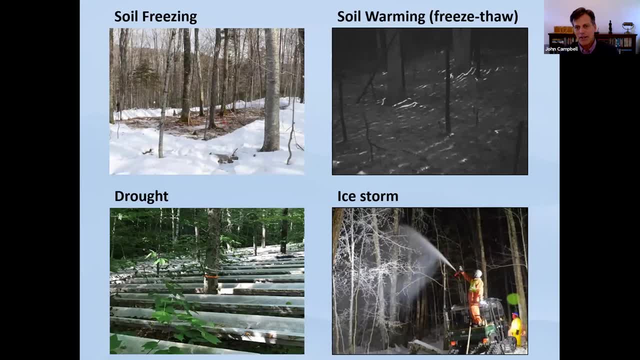 And so there's a lot of mysteries here. We've been trying to understand what's driving these, and for each one of those spikes there have been experiments designed around them. There is a series of soil freezing experiments where, you know, snow is removed off plots and to let the soils freeze, And so this is kind of a blow ground experiment or blow ground. 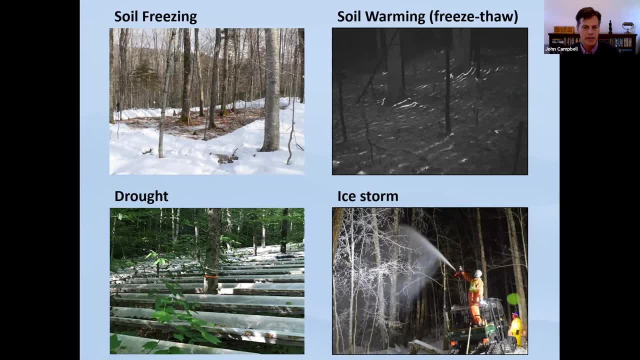 disturbance that affects plant or vegetation and the roots and prevents them from taking up nitrogen. Pam Templer talked in the last webinar in this series and I think she covered the soil warming and freeze thaw experiment that she's been involved in. Heidi Askrodson at the University of New Hampshire is leading a drought experiment where she set up these kind of troughs and have shunted water or precipitation off plots to look at impacts of droughts. 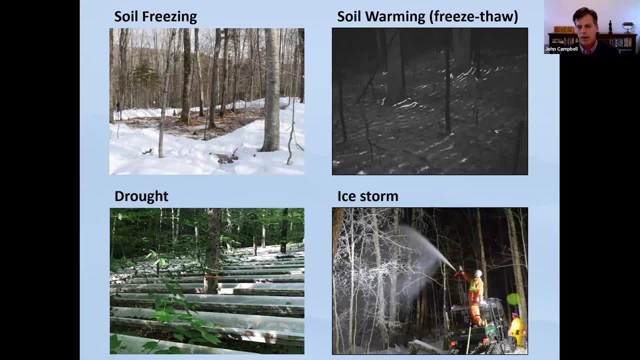 And then, lastly, we've had this ice storm experiment where we spray water above the forest canopy during freezing conditions to kind of simulate a glazed ice event. I don't have time to go into the results of these studies, But it's not always a clear picture, And so but this has helped us try and understand some of the mechanisms that are driving these peaks in nitrogen and stream water. 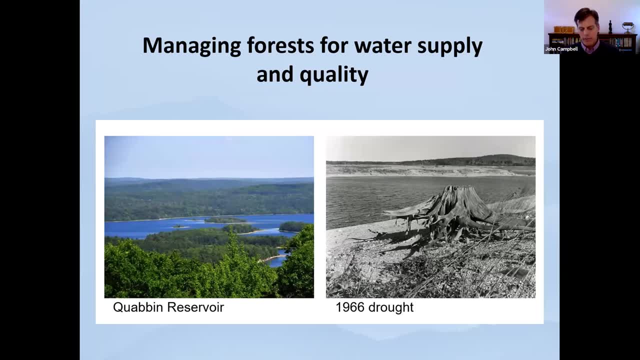 Okay, I want to just end with a few slides about forest management and impacts for climate change and hydrology. In the northeastern US we don't typically manage forests specifically for water supply and quality. It's usually one of the considerations, but generally not the primary considerations. There are some exceptions to that. 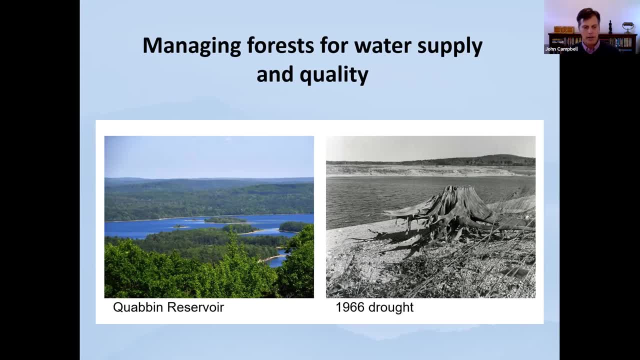 such as maintaining watersheds for drinking water. This is a picture of the Quabbin Reservoir, which is the water supply for Boston, as you probably know, and they put a great deal of thought into how best to manage the land around the Quabbin Reservoir to ensure 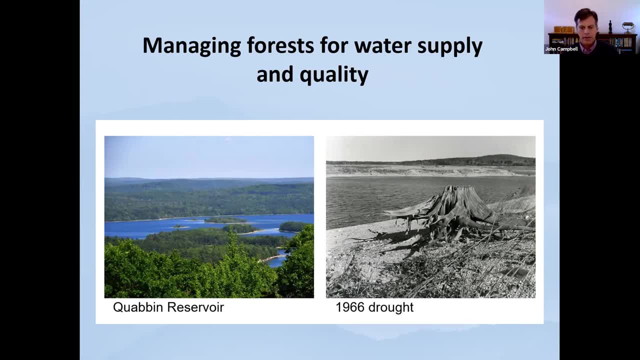 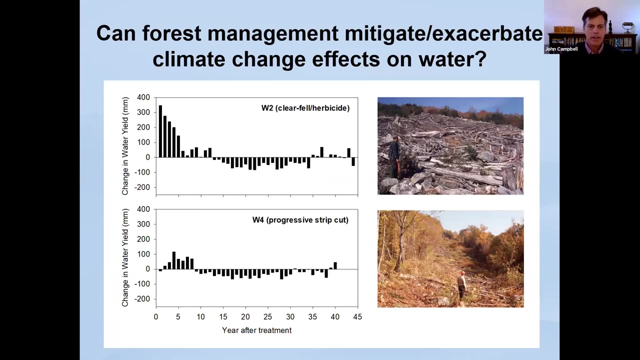 that the supply and quality of water is maintained even during the most extreme circumstances like this drought in the 1960s or the 1938 hurricane. So we don't typically manage specifically for water quality. but it does raise questions about whether forest management mitigates or exacerbates kind of climate change effects on water. 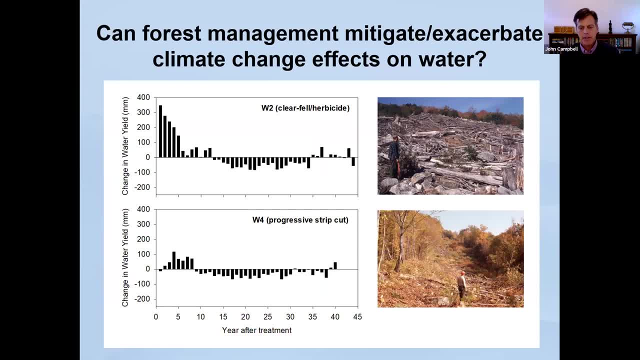 And at Harbor Brook there have been several cutting experiments that shed some light on this. These graphs show the change in water yield following two different kind of experimental cuts. One was a watershed that was cut and all the trees were left in place, and then it was sprayed with herbicide for three growing seasons. 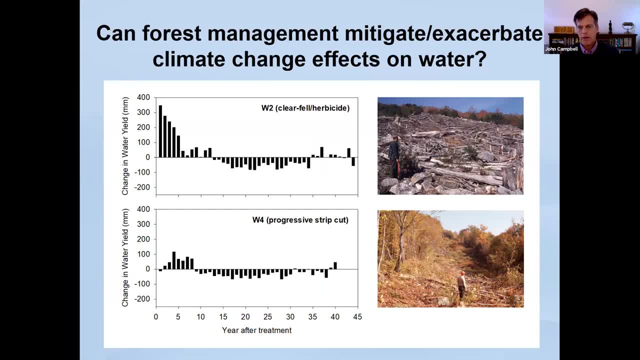 The other one was a progressive strip cut where these 25 meter swaths were removed from the forest. So this is kind of like a gentler type of treatment And in both cases you see this increase in water yield in the years after the cut, but it's followed by a long period of a reduction in water yield. 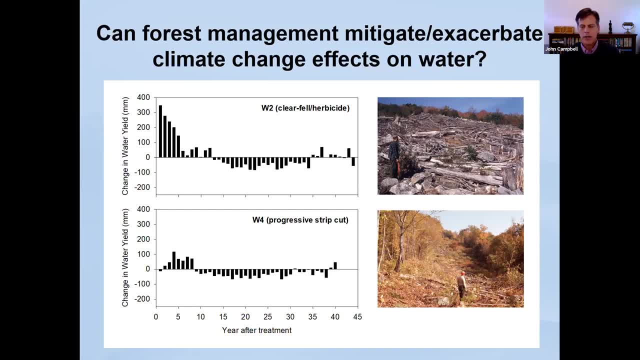 And the reason for that is the first species to move in is pincherry, which has very high transpiration rates, And so it made losses of water via transpiration, And so you know we typically don't manage thinking about water, and you know transpiration that becomes tricky to control over the landscape over a very long time period, And so this is not something we generally consider. 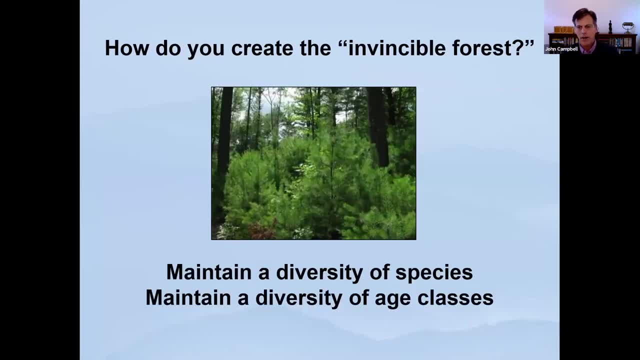 It does raise questions about how to manage forests. for kind of climate change, though, And I you know what everyone kind of wants is this invincible forest, And what I mean by that is one that can withstand that natural and human disturbance and recover very quickly. 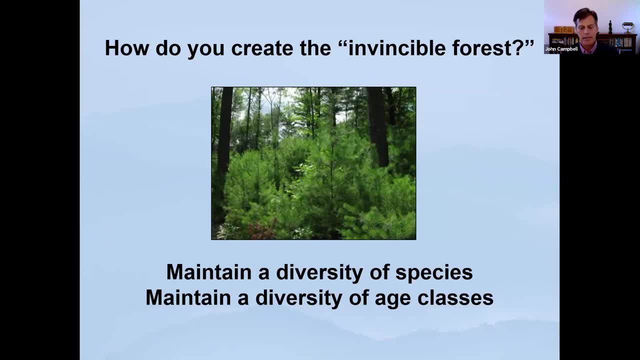 And the way to do that is to kind of hedge your bets by, you know, maintaining the diversity of species and diversity of age classes. This is generally things that people do in general, because it's good for forest management and can certainly enhance recovery after disturbance. 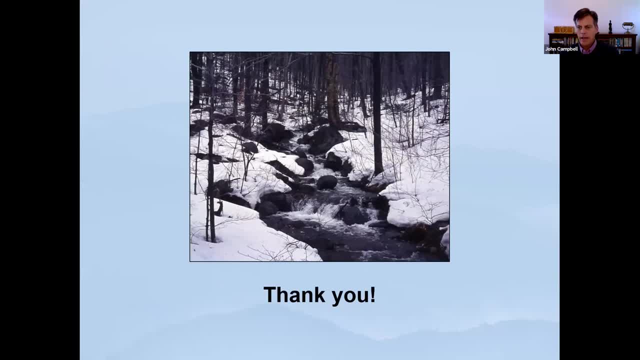 Okay, so I will end there And I guess we'll have some questions to the end, and I'll pass the reins over to Erin Great. Thank you so much, John. Yeah, so we'll let Erin take the floor with her presentation. 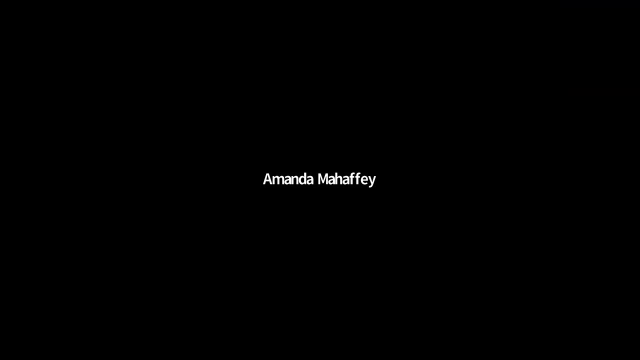 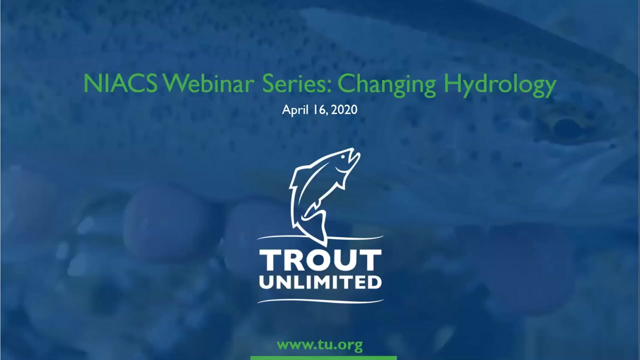 We do have a question in the chat box, So, other folks, please feel free to type your questions into the chat box And once again, we will start addressing those after Erin's presentation concludes. All right, here we go. Hi all, So thanks for joining us today and 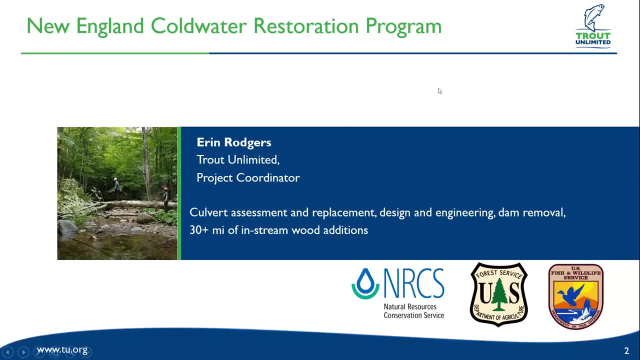 All right, there we go. So I'm Erin Rogers, I am the project coordinator for Trout Unlimited and I kind of cover the range throughout New England, Doing everything from culvert assessment and design and replacement to the in-stream habitat and woody additions. 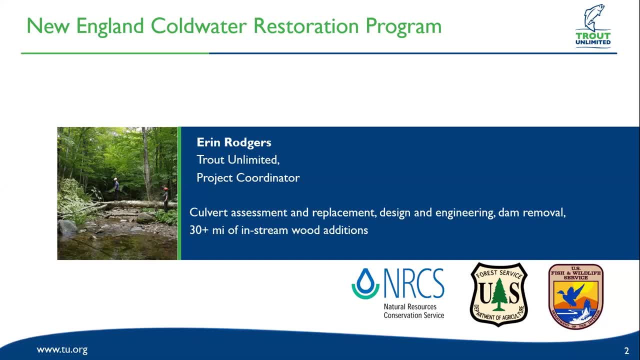 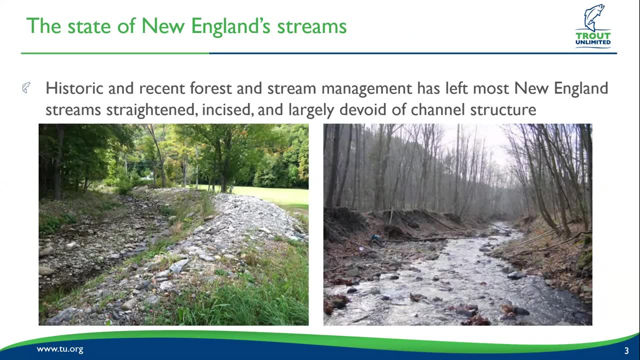 that I'll mostly be talking about today. Just to kind of give a state of streams in most of New England at the moment, you know there have been a lot of historic land use changes and even recent forest and stream management that has left a lot of streams very straight and very much down cut. 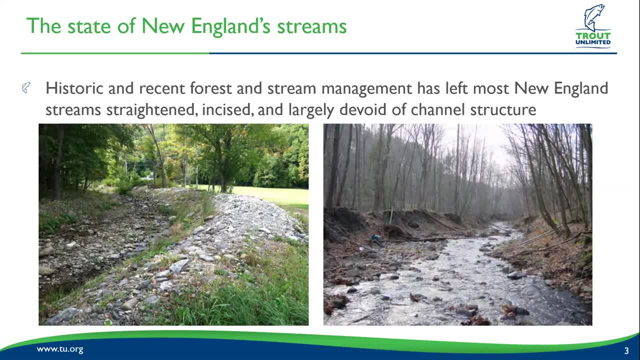 This has a lot of repercussions that I'll get into more and more over time. But basically you know a lot of our, a lot of historic land use changes have you know have all been towards keeping water in streams and very much within those streams, to the point of even building up berms, larger banks and kind of shuttling water as fast as we can onto somebody else's property. 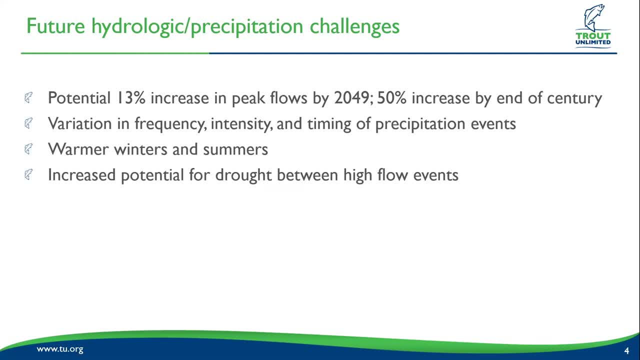 As John's presentations were saying, you know, the peak flows and average flows or peak rainfall events, average rainfall events, which obviously lead to peak flows, have really been increasing over time and projecting out into the future. some modeling that has been done recently by both Richard Palmer, Keith Nislow and many others. 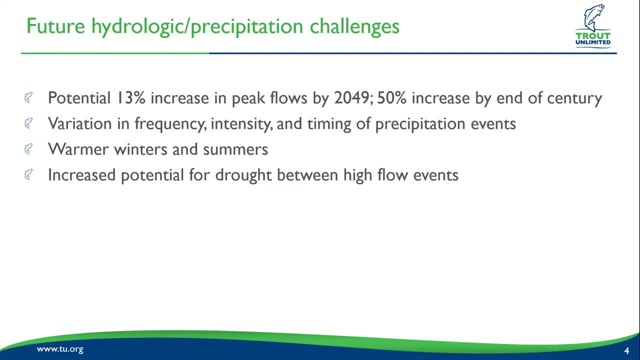 has been, has been showing that, you know, it could be up to a 13% increase in peak flows by mid century and up to a 50% increase in mid flows by the end of century, which is a lot of water to account for spatially. 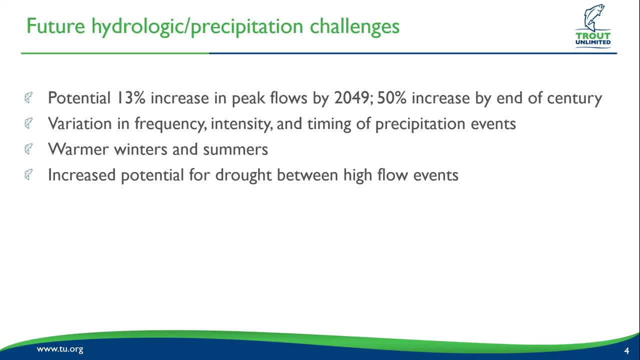 The variation in frequency and intensity has really been changing, as a lot of John's graphs showed: not just higher highs but lower lows between those warmer winters and warmer summers, with increased potential for drought, between these high flow events. So things that I have to end up. 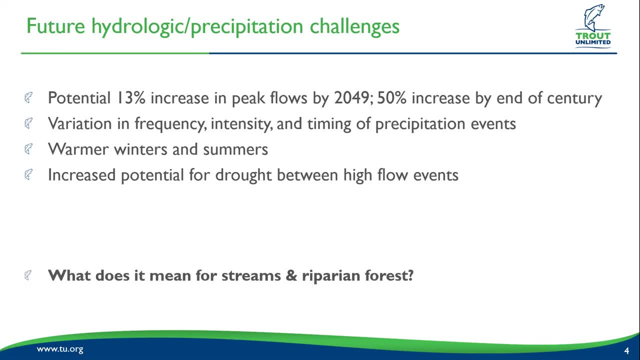 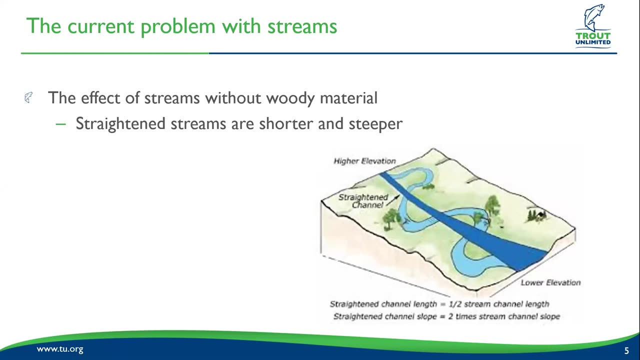 paying attention to both sides of that when I'm looking at fisheries And really what that again means for not just streams but for the riparian forests surrounding them as well. So stream channelization: most people don't really think of it terribly much. 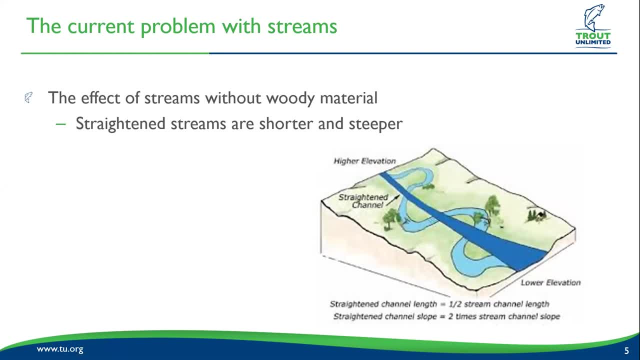 But really a straightened stream is a shorter stream and covering the same amount or covering less distance down the side of a mountain or down the landscape, But still covering that same elevation drop, means that we're also seeing a lot steeper streams. The flow is, you know, very much impacted by this nice shooting shuttle of water coming down the mountainside. 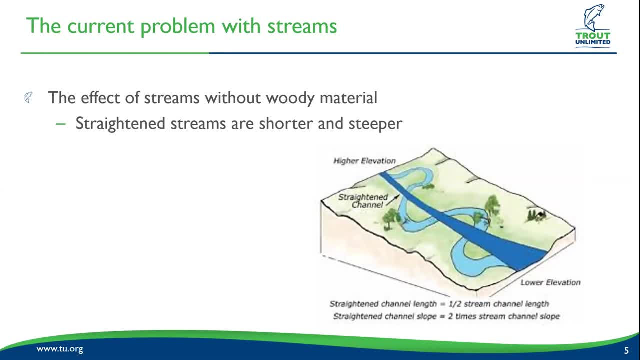 But also, when you're talking about shorter streams, You're also changing the volumetric capacity of those streams as well. So a longer stream, you can store more water in it over that same distance than you can the shorter stream that now exists there. 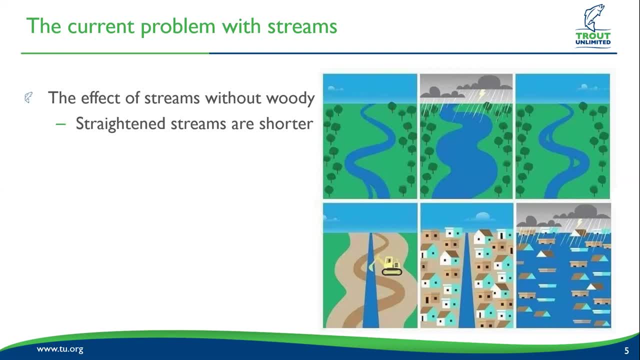 And that kind of shown through this graphic that I stole from another paper. You know you've got the more sinuous channel- doesn't nearly flood out quite as wide as you know- a channel that has been straightened and run straight through a town, both from 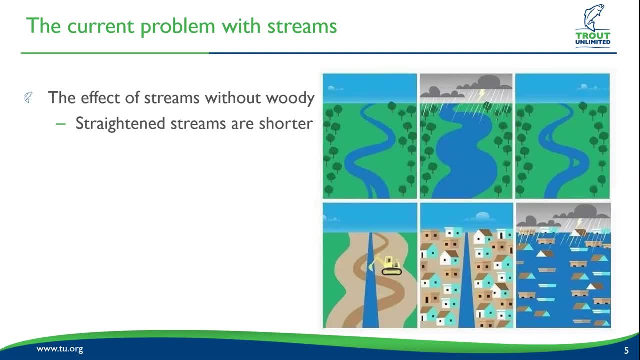 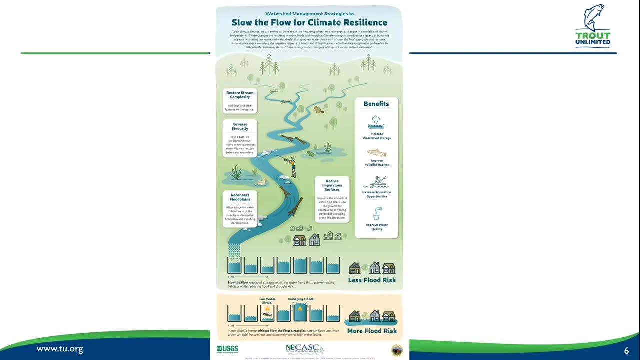 You know the lack of or the changes in porosity from the surrounding landscape, but also just because you can't fit nearly as much water in that channel as you once could when it had that sinuosity built into it. Another wonderful graphic stealing from another group, from the Northeast Climate Adaptation Science Center, out of UMass or out of Amherst: 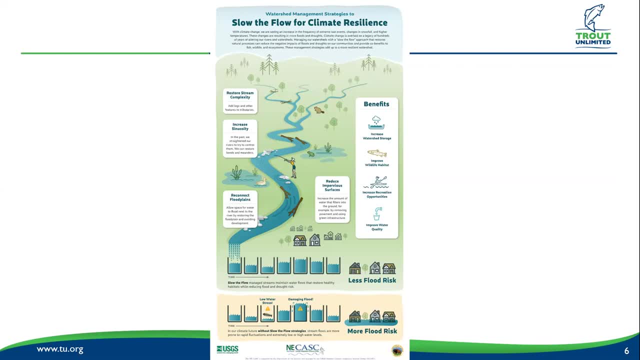 Getting to some of these points in a very nice simple graphic That's really highlighting their work to to find ways to slow the flow so that you know finding alternate ways of storing water in those upstream forested watersheds before they really are able to impact the human communities on the downstream end. 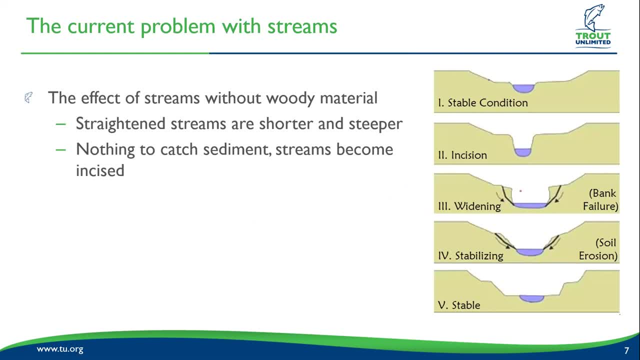 With the increase in floods, increase in peak flows It has that water has more capacity to move larger objects out of the stream channel. So it's pushing the large what out is pushing the large boulders out, and people are having a really good time helping that along as well. So without 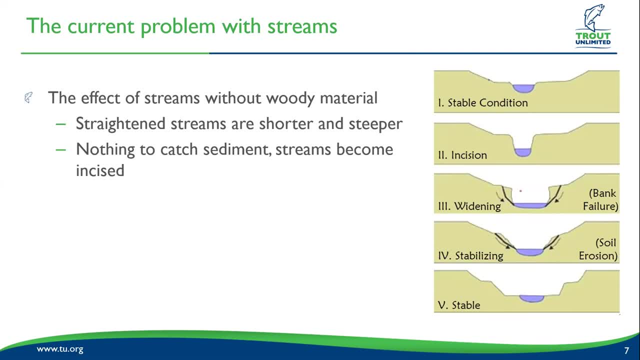 You know, objects without structure in the water There's really nothing to catch the sediment and it cuts down in the channel. So if we started off historically 150 years ago in the kind of stage one, stable condition, you know, over time channeling, more flows, higher velocities. 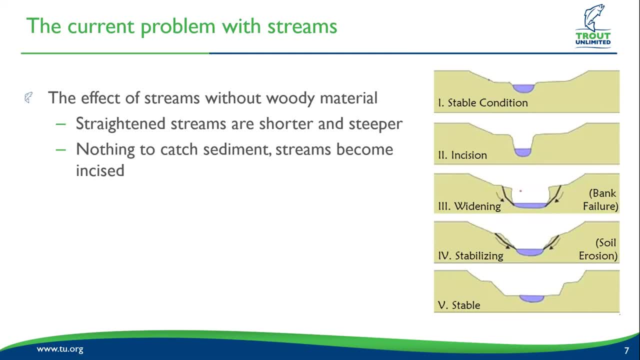 We work more and more into the kind of stage two incision. so stream channels are cutting down as sediment is being worn away. That leads to instability and the banks start to fail. streams get very wide, streams get very shallow. It starts to stabilize a little bit after that and basically hits a secondary stage five: stable condition. 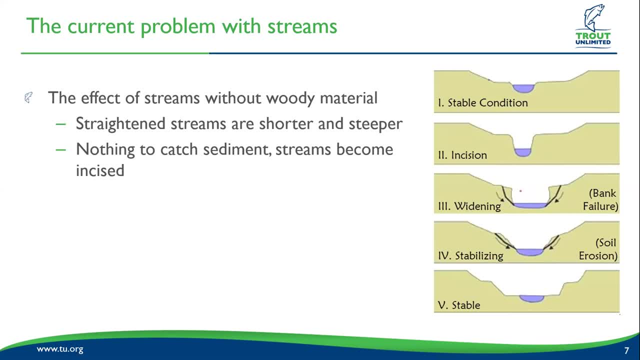 But it is substantially lower elevation than previously. So most of New England is pretty much in a stage two and stage three through most of our streams, especially our headwater streams, And you can see that in, you know, if you, if you just drive along the roads. 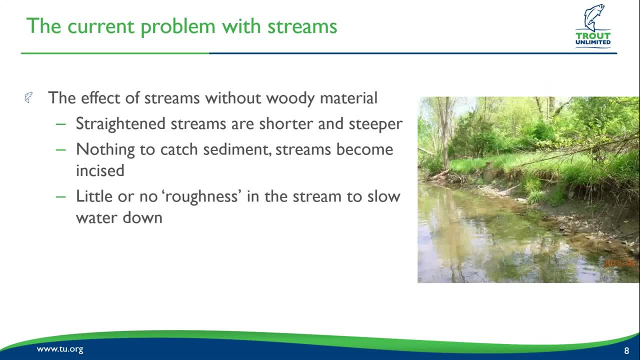 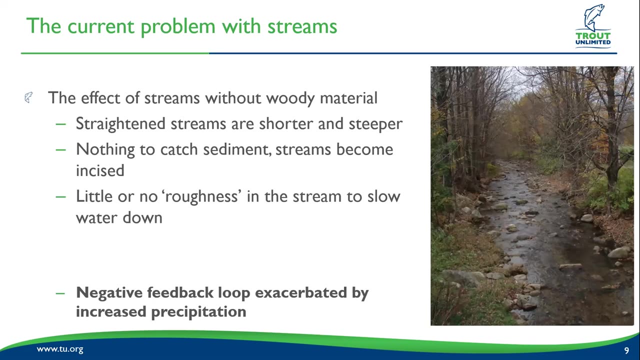 A lot of things you'll see through there And again, with little to no roughness in the stream. There's not a lot to slow water flow down, And that kind of leaves us with a bit of a negative feedback loop that's just increased by, or exacerbated by, that increased precipitation that we've been seeing across New England and across a lot of the northern tier of the states. 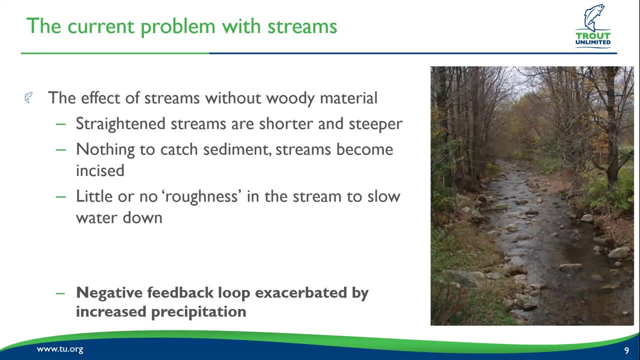 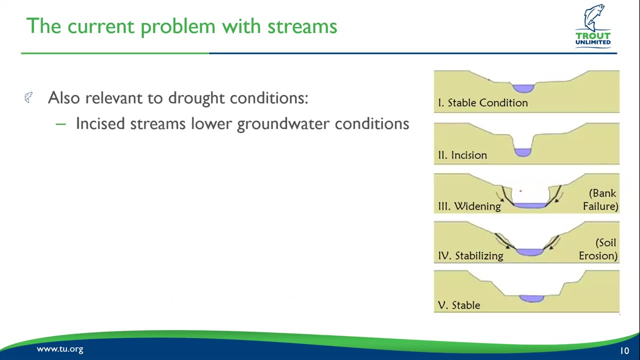 Higher flows, more erosion Through the stream bed. you get more incision, more widening and it just creates that same process over and over again. And this is also relevant to drought conditions. So when you have an incised stream channel, it lowers that kind of baseline groundwater condition. 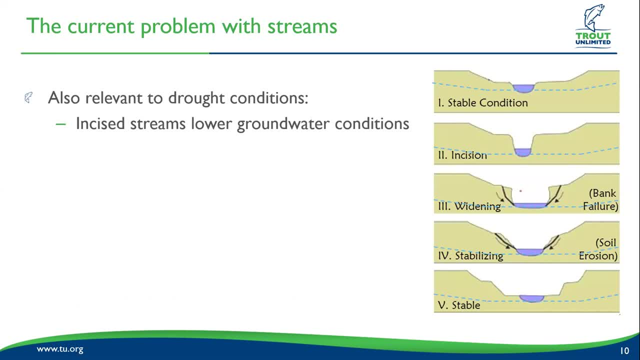 So again, the historic stage one. you've got a higher groundwater table as it cuts down through incision and through widening your. Your groundwater table, both at the stream level and in the surrounding riparian forest, has been cut down, you know, two to three times, depending on the severity of the incision. 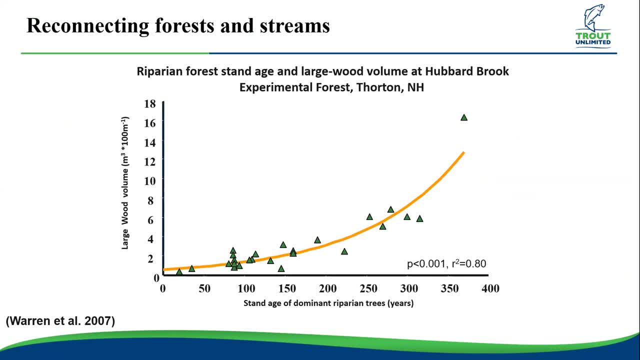 And that really leads to How we can reconnect the forest systems and the stream systems. I feel like there's been a lot of years that they've kind of been separated in terms of theory and practice, and We're kind of just now kind of coming back into how we can reconnect these things. 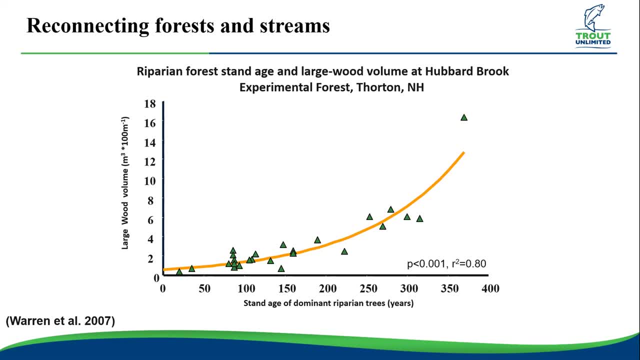 So this is a chart from Warren's paper back in 2007. So looking at the age of the forest stand versus the volume of large woody material in the stream channel, obviously young forest. There's very little In stream wood in the channel And as you get older and start to get into those old growths, forests. 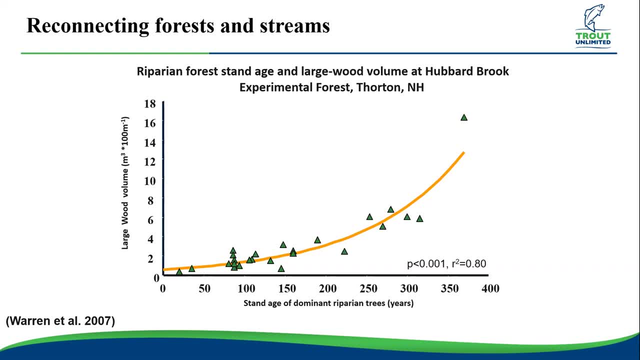 The amount of wood in the stream channel really starts to increase. Other modeling done by Keith Nislow has shown that, or has Kind of been modeled out to optimally. in old growth forests and mature forest you would see anywhere from 270 to 320 pieces of large wood in a stream. 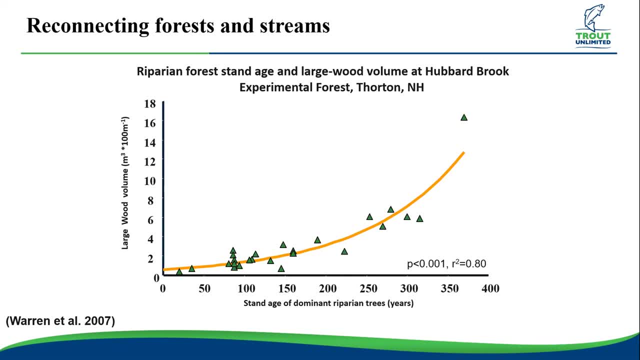 Per mile and By most counts, even through, you know, protected lands, national forest lands, We're seeing on average maybe 10 to 20 pieces of mile of large stream per month, of large wood in the stream per mile. so There is there's a big gap in what we are seeing currently with what could be there in a healthy stream system and stream and riparian system. 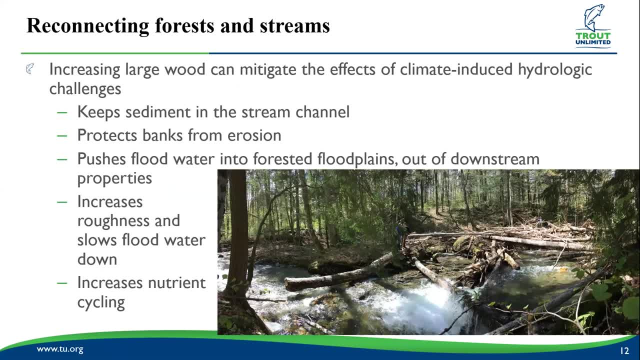 Increasing the large wood in streams can mitigate a lot of the effects of climate induced hydrologic challenges. So it's helping to keep the sediment in the stream channel, protecting banks from erosion. It helps to, you know, push that floodwater back out into the forested floodplain. 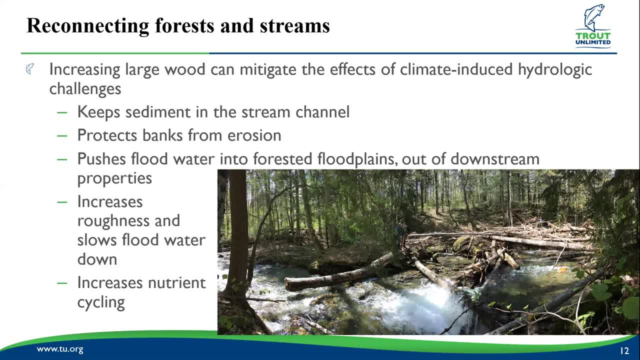 It increases the channel roughness, It slows the floodwater down, creates hydraulic velocity barriers And even over time, just during normal conditions, It's been shown to help increase nutrient cycling. So those problems that we're seeing with nitrogen, with phosphorus and different water bodies, 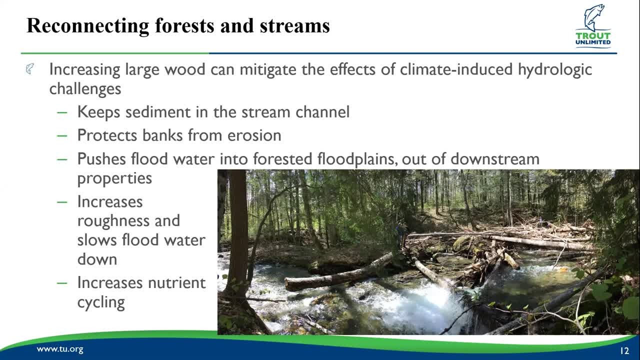 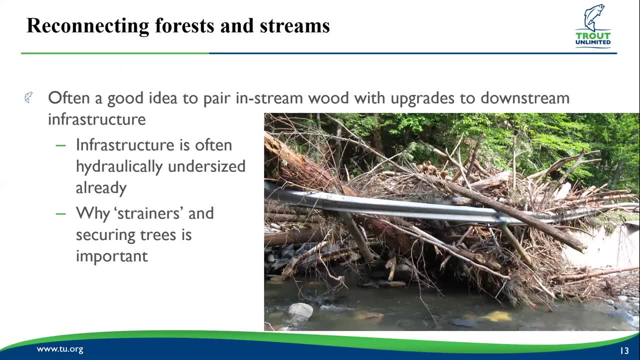 Not that this is a hundred percent cure all, but it can certainly be a piece in the larger puzzle And it's really good idea to these kinds of in stream large with projects with upgrades to road stream crossing infrastructure. Just like to note that in the picture here that was not caused by any kind of large in stream would addition. 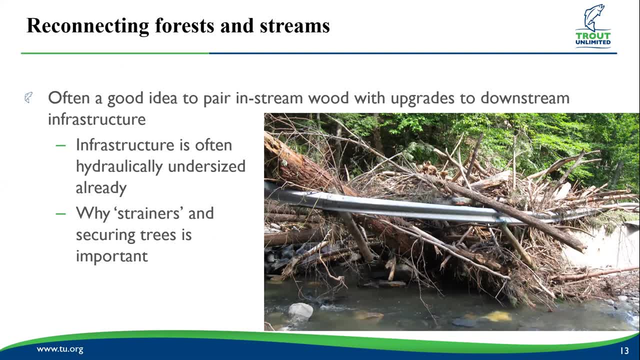 That was actually from a picture in Western Massachusetts after Hurricane Irene. So this is just stuff that was coming off the landscape anyway. But what I have found through a lot of my corporate work is that in any given watershed, sub watershed, Roughly half of all road stream crossings are in stream. 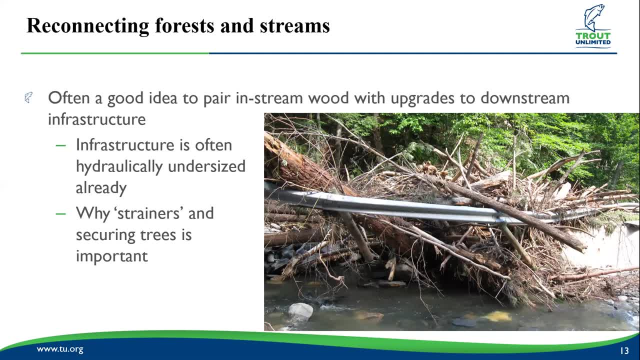 Crossings are either moderately to severely undersized for the stream channel that is flowing through them, The cost of doing of doing these upgrades is pretty substantial. If you're working with town and state roads, you can get away with a lot more flexibility. 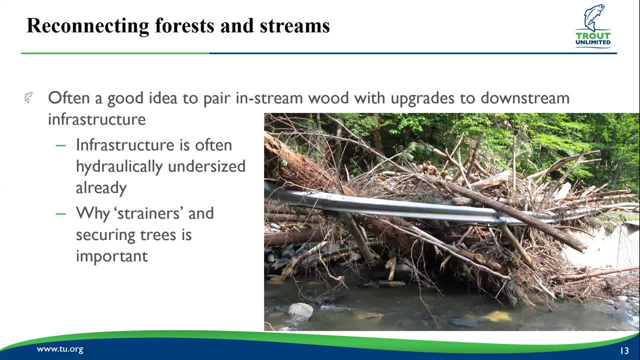 If you're working on forest roads, harvest roads, especially if it's temporary bridges that you can then take out from you somewhere else for another year And in kind of the large woodwork. This is why we use a lot of what are called strainer trees before we get anywhere near infrastructure. 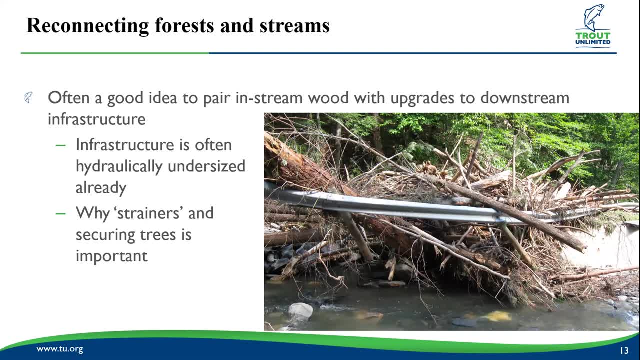 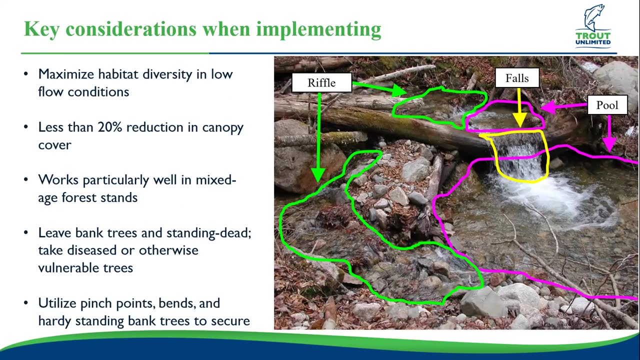 And the importance of securing a lot of the trees in kind of the different ways that we use, methods based on the size of the streams that we're working in. So, again, some of the key considerations that we're looking at when we're implementing this, being a fisheries person for Trout Unlimited. 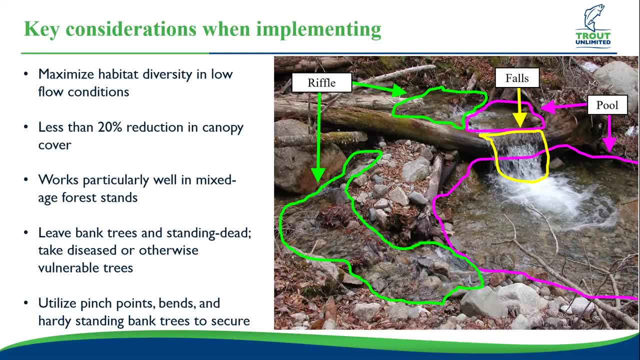 We're really looking to maximize habitat diversity, both in normal flow, low flow conditions and kind of keeping things in in place during those high flow conditions as well. When we're working in any given place we're aiming to, you know, we're not opening up the canopy cover any more than 20% and that's, you know, at a at a maximum. usually it's a lot less than that. 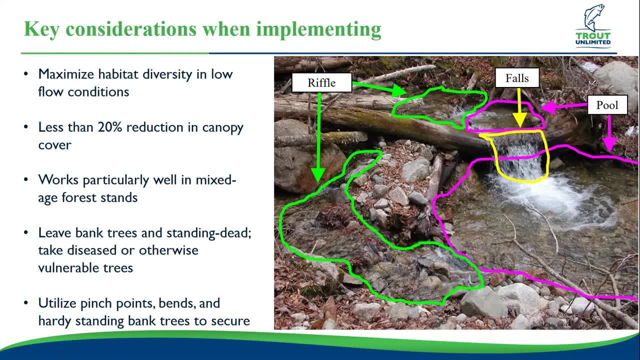 The kind of works that I'll be showing In the next few slides work very well, But we're also looking at really mixed age forest stands That way, when we're using some of the mature trees to, you know, put into the stream channel. 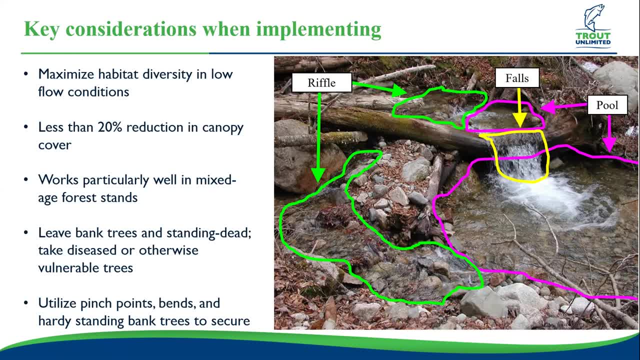 There are those younger and middle aged trees that can easily and pretty quickly fill in those gaps. We always leave bank trees and standing dead trees because they're wonderful bat and bird habitat and more and more lately over the last few years, we have been taking disease trees and otherwise vulnerable trees. so starting last summer we've been 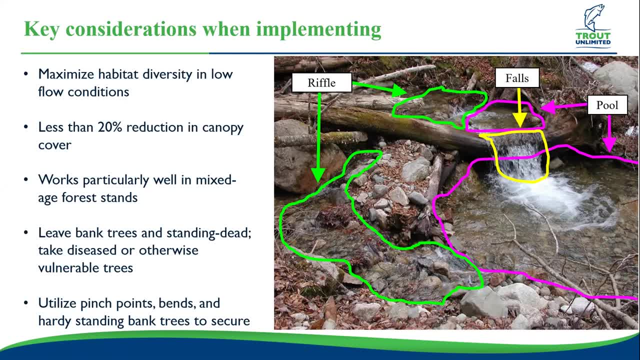 taking a lot more of the white ash in anticipation of the Emerald dashboard that's been, you know, making its way up through Vermont and the rest of New England. And we also utilize pinch points and natural bends in the river, finding ways that we can help emphasize those areas and using those standing bank trees to help secure wood in place so that it's not becoming a risk to downstream infrastructure, to downstream landowners. 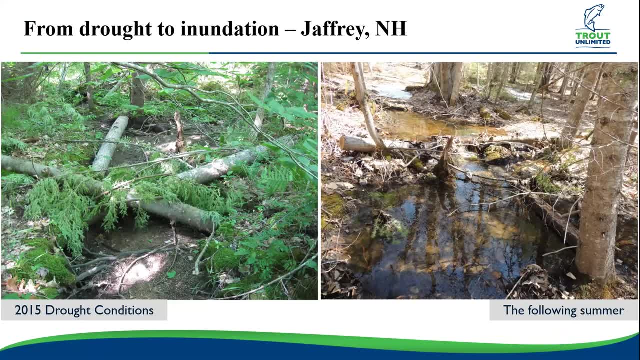 And so just a few examples of some of those. And so just a few examples of some of those. And so just a few examples of some of those. So just a few examples of some of those, Some of these things. Back in 2015, we were doing some of this work, and it was That was one of the pretty substantial drought years, such that we were working in a lot of channels that didn't have water flowing in them at the moment, so it was a bit of a guessing game as to wood 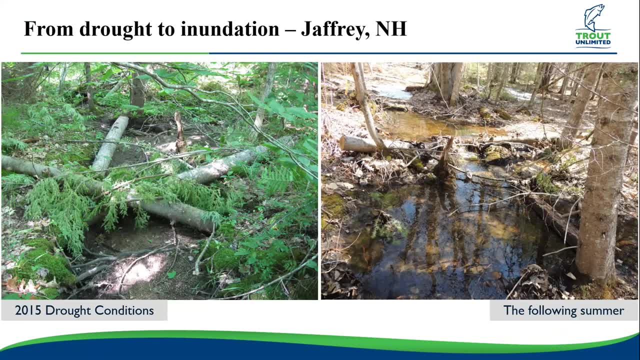 placement. But you can see here from a project site in Jeffrey, New Hampshire What this kind of smaller installation has been able to produce on the upstream side, produce on the other side in terms of pushing water out to the edges and kind of creating more of a braided channel, more of a little bit of a floodplain. 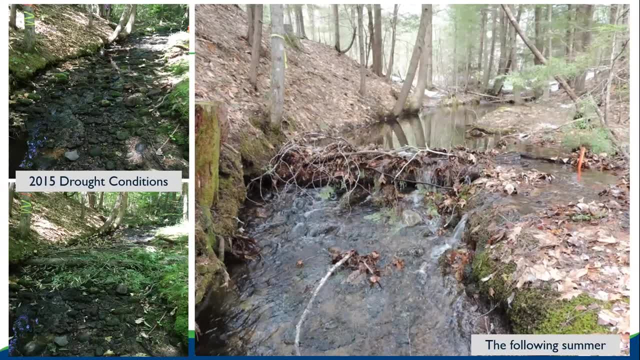 access through here, Another site from Jaffrey, again a nice straight, very wide channel and then the following summer. so that's just all material that once water did start flowing through the system again and through the fall, collecting small woody matter and leaf litter kind of fills in those gaps and brought 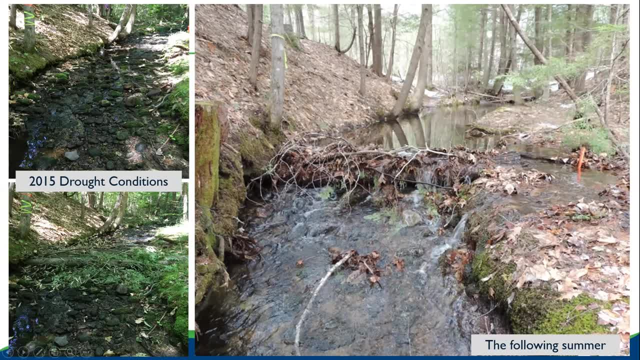 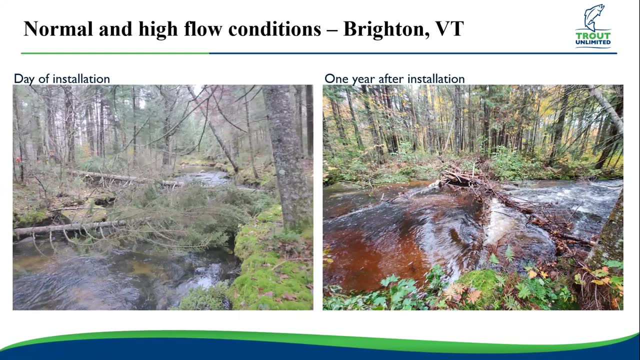 the stream channel basically right up to its banks instead of where we can see the more incised channel on the downstream end still, And it's not always pretty, especially on the bigger streams, right after installation but really quickly the stream really integrates any large wood that we add. 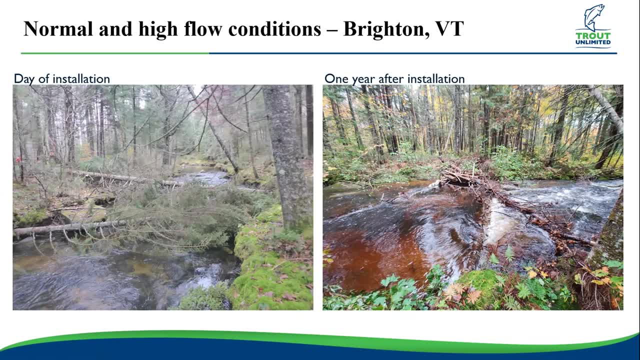 into it very quickly. You can see where these larger hemlock and trees have. you know they've lost their bottom branches, they're sitting farther into the bottom. and the difference between the water flow upstream of the installation to the water flow downstream of the installation. 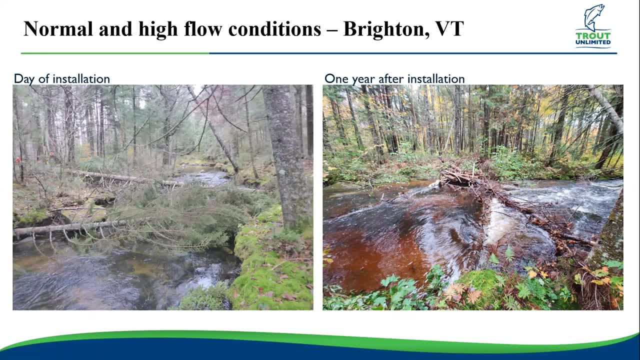 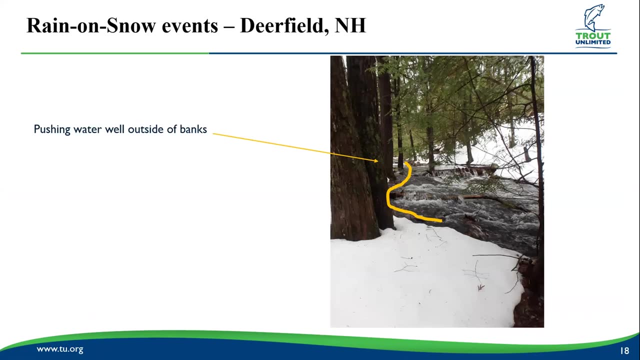 it's significantly reduced. It's also obviously pushed out. it's beyond the banks here, kind of spreading that flow and mitigating the effects. John had talked about rain on snow events and how those. there's a good chance that those are gonna become more and more likely. This is exactly an example of that from. 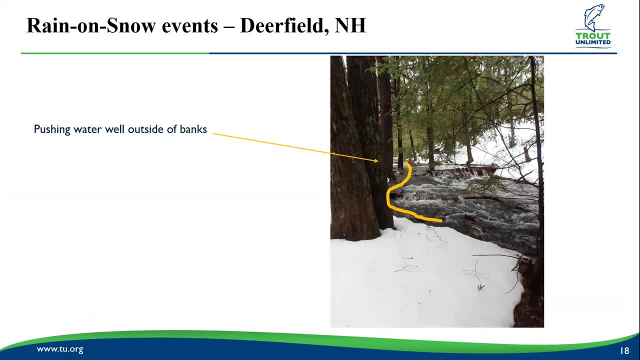 Deerfield, New Hampshire, out towards the seacoast, where we had done several installations- and I think this was the winter or late spring of 2016- on a couple of tributaries to the Lamprey River, And you can see where these installations already are pushing way. 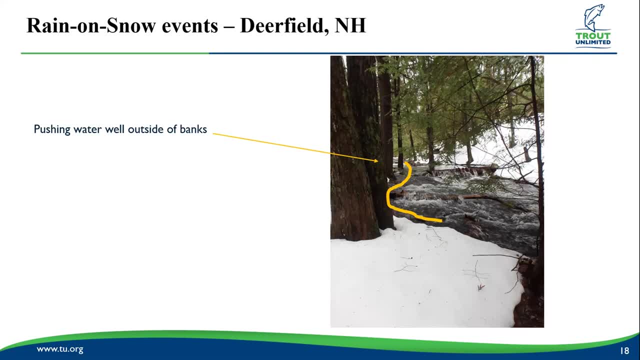 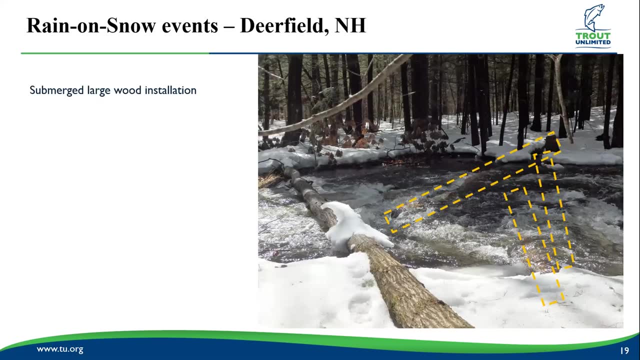 outside of the banks and kind of again creating those nice step pools, creating the, the area available for overflow. One of the further upstream or one of the further downstream sites here, an installation of three or four pretty substantial sized trees, are fully submerged in the river, and you know, 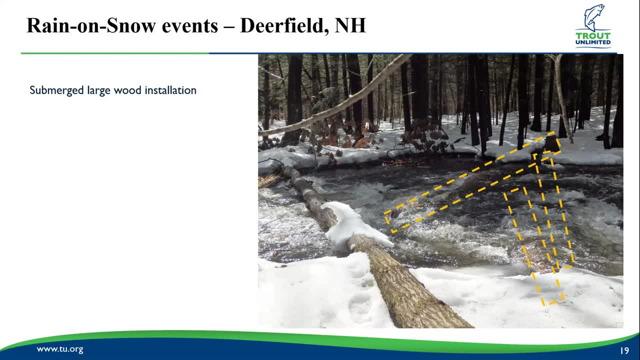 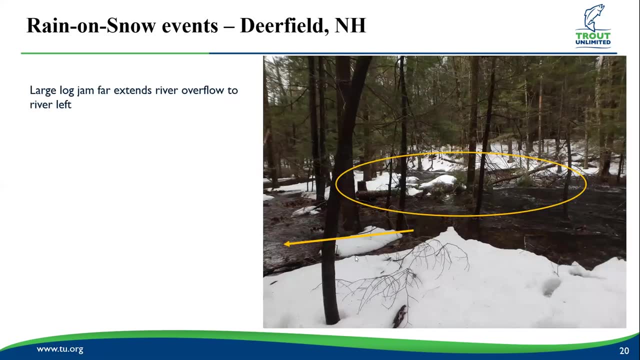 again pushing out, helping slow that flow down, creating those that hydraulic disruption, And then in this one further downstream where it starts to get to be a pretty substantially sized river, this log jam here has created a massive overflow, channel out through the forest to to river left here. So the main part. 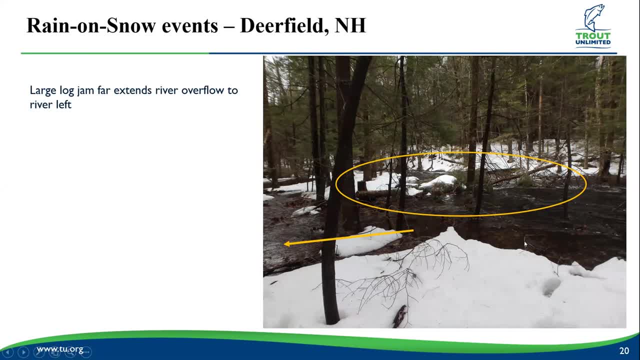 of the channel. the original banks kind of cut this way And the water in the channel at this point is about three or four feet deep. But there's this, you know, fairly large swath cutting down around and through the forest And, as winter, rain on snow. 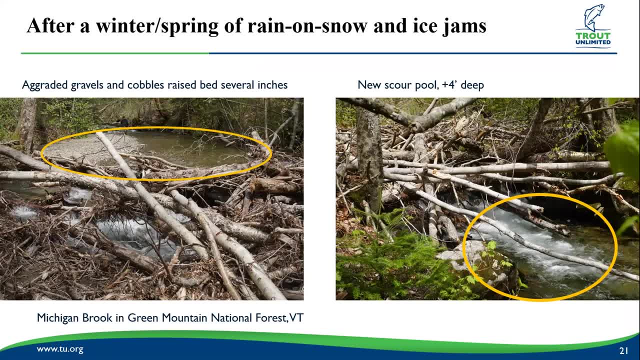 events become more and more common, or rain on snow events become more and more common and ice jams and ice damming becomes a problem. So this was at a site in the Green Mountain National Forest Where you know this was less than a year after installation and wound up. 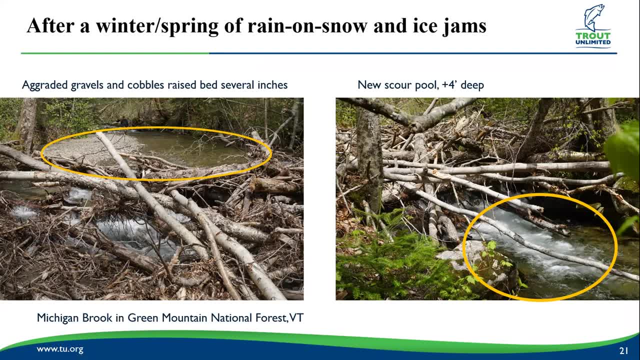 having a very severe winter and a very severe spring Where several of the smaller installations ended up kind of amassing into one very large log jam Which luckily, with the Green Mountain National Forest, we have the flexibility and the latitude to have really big messy jams like this. Not every landowner. 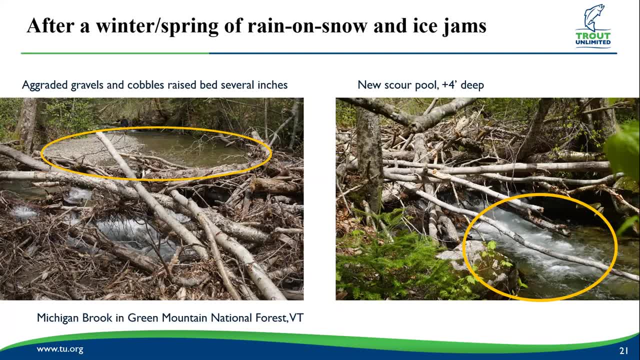 uh, would, would you know, find this nearly as acceptable as the Forest Service does? But they were. they were pretty pleased by it And one of the things to really pay attention to in these two shots. this is the same jam, kind of looking upstream. 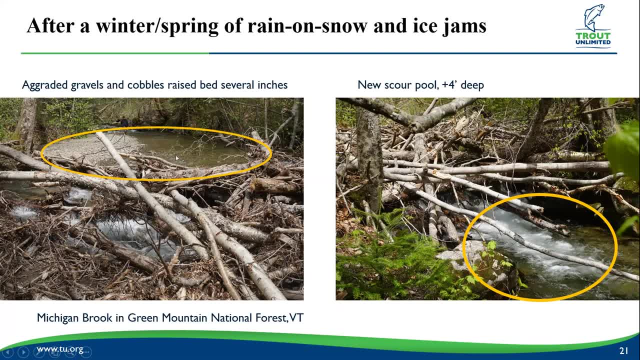 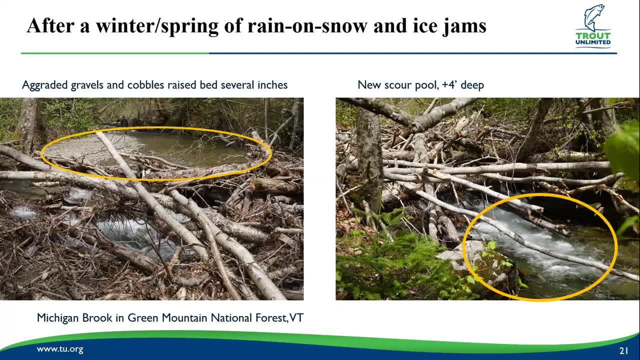 conjunto ofontnormal streams up here. But when you go down the water slide- freaking deep down, float Power descending down the lower bottom usual standard- there is about a foot and a half of difference And the scour pool that's formed on the downstream end is four or 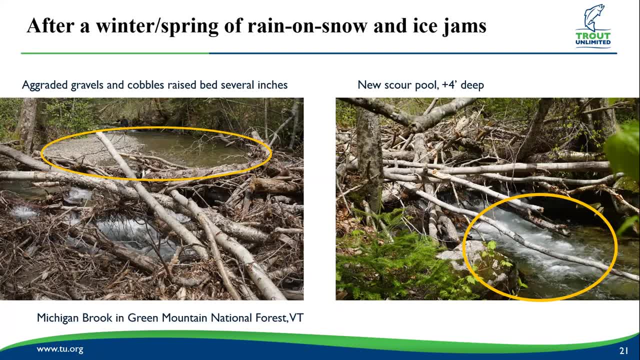 more feet deep right there, Which is incredible habitat for a lot of cold water species, As we're talking about warmer winters and warmer summers, you know, in streams that are less groundwater influenced and more influenced by the air temperature surrounding. uh, having that, those 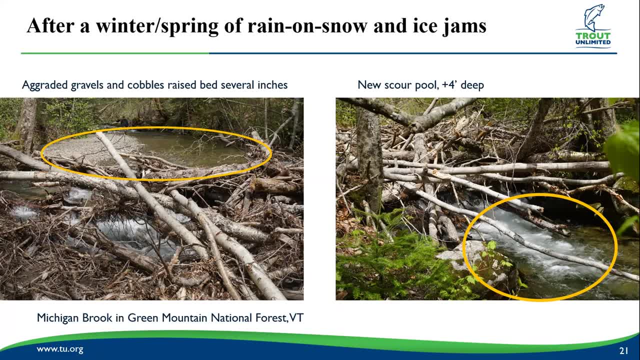 nice. deep pools as cold water refugia for our cold water species is incredibly important, And these kinds of large wood structures are actually a lot more porous than they look. Yes, there are several feet difference between, you know, stream bed upstream and stream bed downstream. 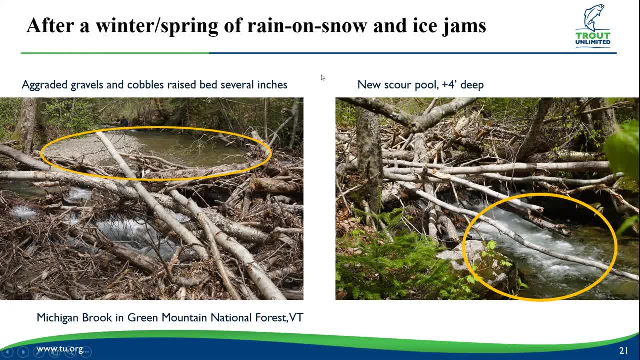 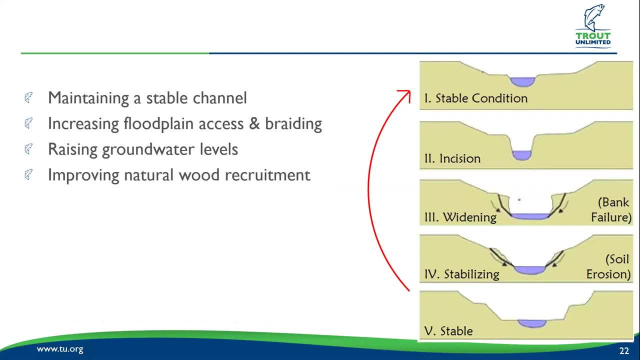 but that's still very much a passable structure if you're a fish. So really what we're doing with this kind of work is bringing it from the kind of more incised stage five stable condition back up to a more graded stage one stable condition. So 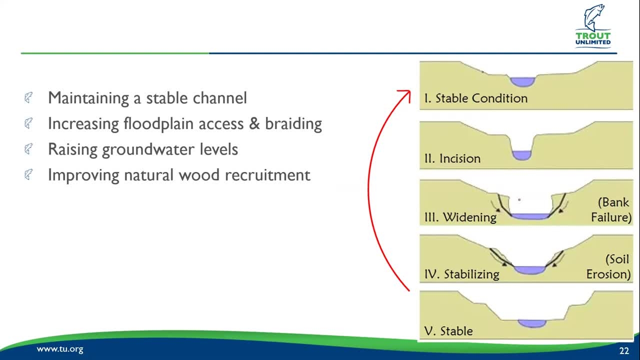 trying to bring these stream beds and stream channels back up to have that easier access to floodplains, to have that easier access out to the riparian forest, It increases that, that floodplain spread and then it's just you know, it's, it's, it's just you know, it's, it's you know. 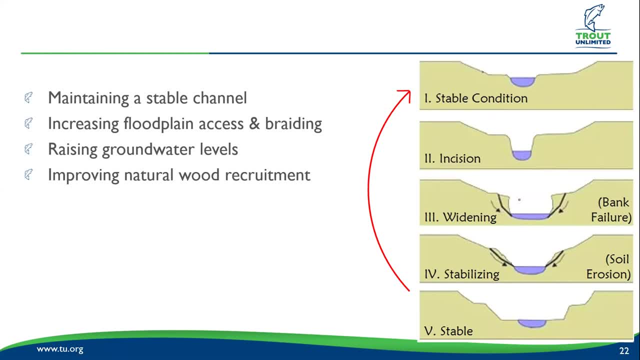 increases braiding in a lot of places and it helps kind of raise that groundwater condition back up as well so that hopefully during those times of drought that we do see that there will be less forest stress on those trees if the groundwater table is a little bit more easily. 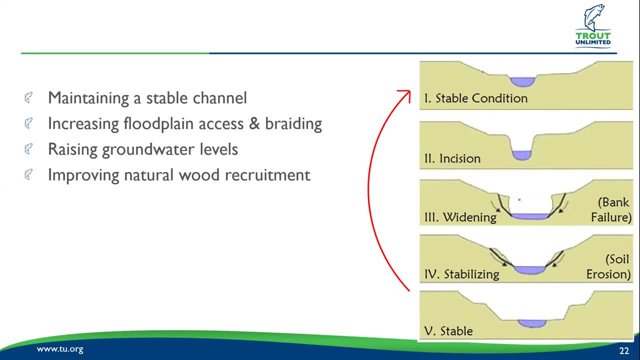 accessible there And it also improves natural wood recruitment. This is a lot of kind of adding. the large in-stream wood is just kind of re-kick-starting that process. So we don't expect it to be stable forever, but we do expect it to be able to be replaced by. 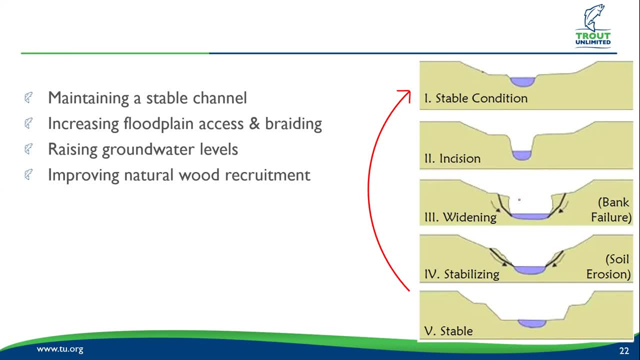 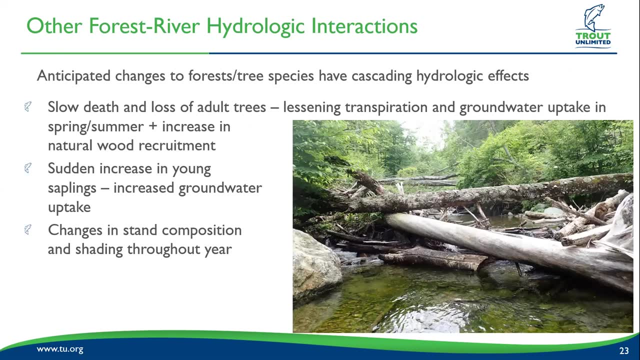 the natural pieces of large wood otherwise coming into the stream. And when we're doing this kind of work there are plenty of other forest and river hydrologic interactions that, not being a forester, I always kind of think about but never really have the you know. 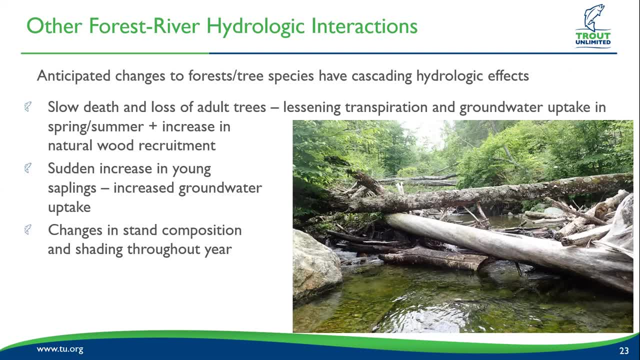 capacity to study, I guess. So I mean looking at all of the literature. you know there are going to be changes in forest types and that we're going to lose certain types of trees entirely, So that slow death and loss of adult trees, you know, leading to changes in transportation and groundwater. 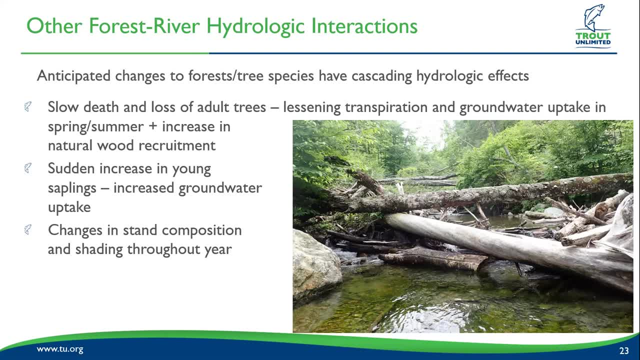 influence. it also means that there's going to be a lot more natural recruitment, like those wood seen in the picture here, And then after that there's going to be that sudden increase in young saplings, Whether that increases groundwater uptake, especially if it depends on which species are coming up next. 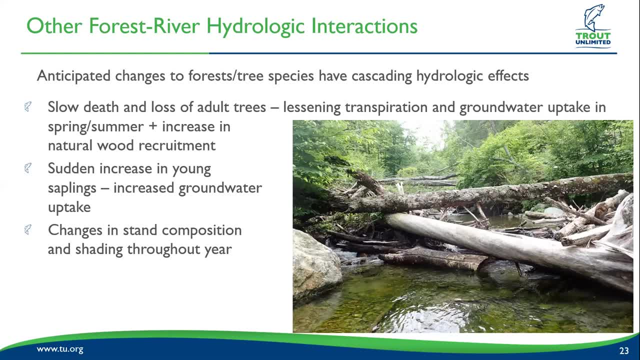 Whether it's. I mean, I probably don't work in a whole lot of areas where pin cherry is terribly common, but you know, the thickets of beach stand that are coming up I can't imagine are not influencing the surrounding stream. So lots of things to think about as temperatures change, as 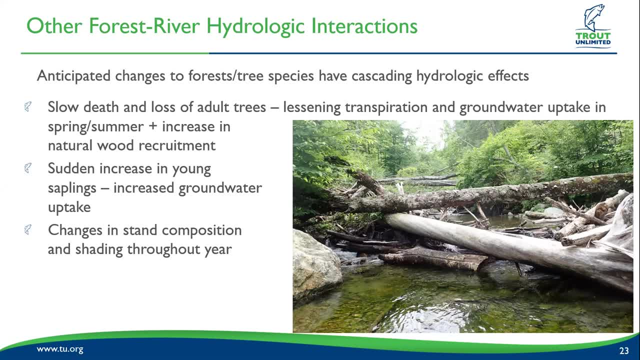 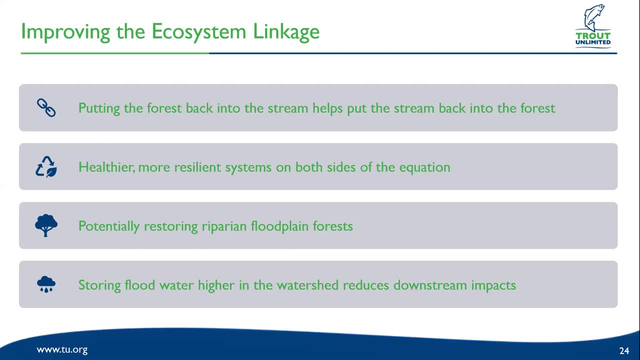 forest stands change, disease and pests come in and interact well with all of this. So kind of the the larger take home of all this is really looking back to that ecosystem linkage of the hydrology, the forests and the streams, kind of. you know we're working to put the forest back in. 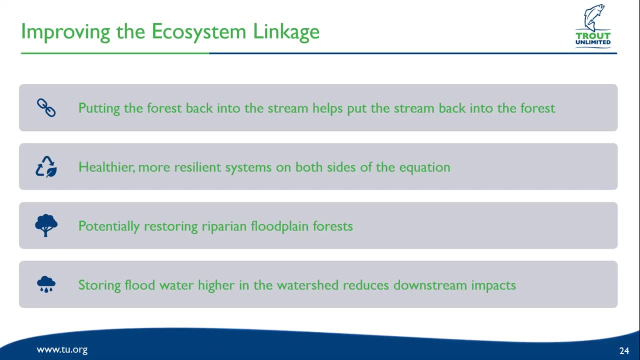 the stream, so that the stream can come back out into the forest as well, And that creates healthier and more resilient systems on the ground. So I think that's kind of what we're looking at right now: More resilient systems on both sides of the equations, Potentially restoring riparian floodplain. 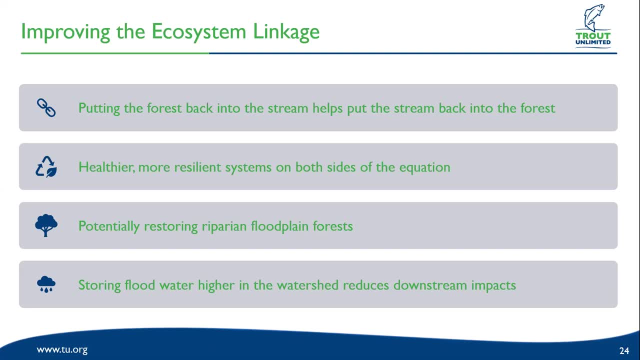 forests that have been diminishing in recent years. It also helps to store a lot of this floodwater higher in the watershed and reduces that impact to downstream communities. So, yeah, that's about it for me. I've seen the chat box popping up pretty regularly, so I'm assuming 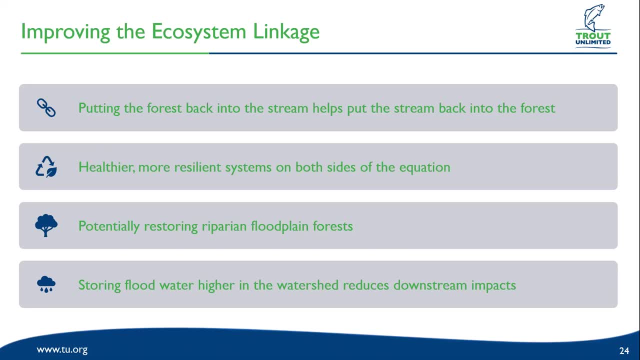 there are questions to be had. Great Thank you so much, Erin. Yeah, we have had some great questions come in, and thank you both John and Erin, for your presentation. We have questions that are for both of you. I'm trying to organize it a little bit. First, for the good of the recording, I want to highlight James Schmierer. 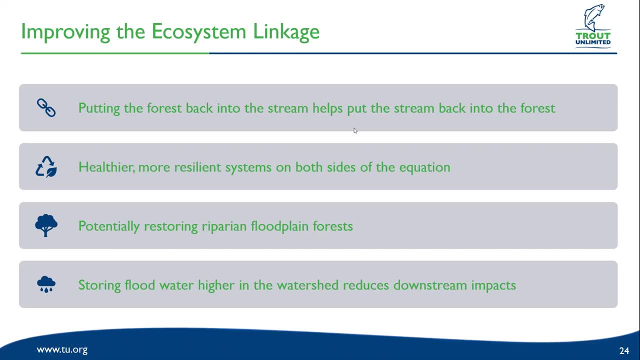 had a question which Maria answered with the publication. Jim asked: has the cost of upgrades and improvements for forest, road and trail infrastructure to accommodate the tire peak flow- is an extreme hydrologic event- been determined and documented? And in the chat box Maria shared a link to a publication that might help answer some of those questions. 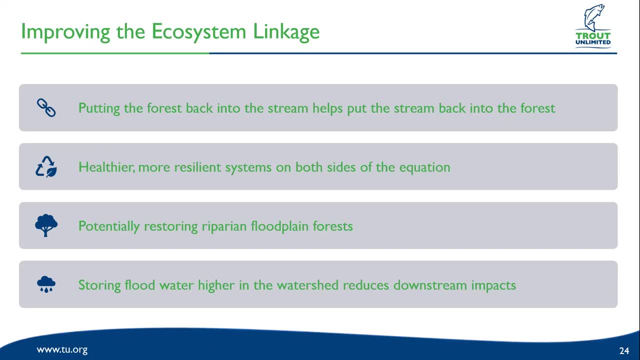 In the interest of time, I'm going to move on. I know our speakers may have something to say about that, but let's see if we can move on for the moment. Another question that was answered. Dominique asked: what is the species with high transpiration rate that regrows after? 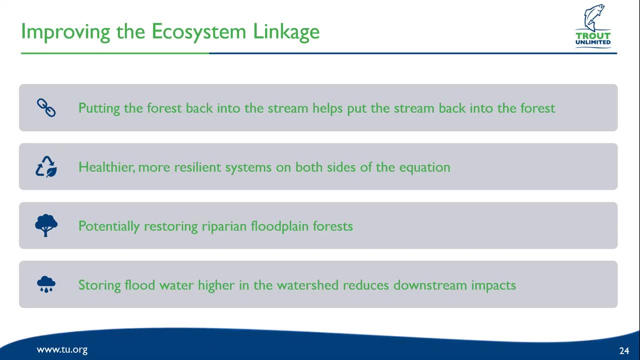 disturbance and pin cherry prunus pezzelbanica was the response. So Jenna Masters wrote in from Hawaii and she says we've been doing a lot of cutting of non-emittered trees and we're not going to be super soakers of water. Is it possible that we are releasing more water into the area? 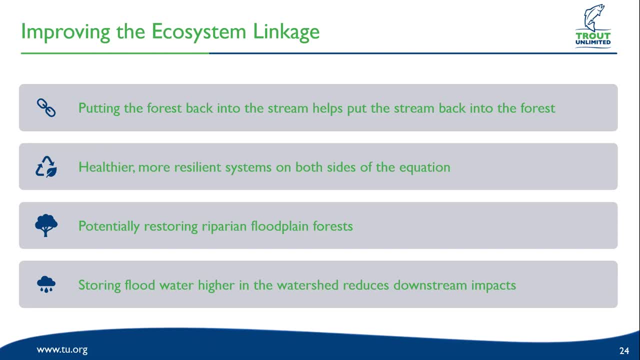 It is one of my theories as to why some of our reintroductions are doing so well- And Tim chimed in as an irony. in the southwest we've been removing ferro types to increase stream flows and raise water tables to good effect. Most are invasive, So John might have something to say about that. 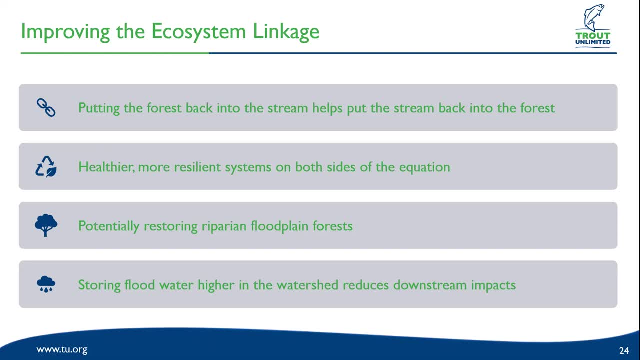 the cutting of non-native trees and what does that do to the water table? Yeah, I mean, I think that is interesting comparison between the two sites, and you know, the species that comes to mind for me is tamarisk in the western US, which people have been trying to remove for years now, and you know. 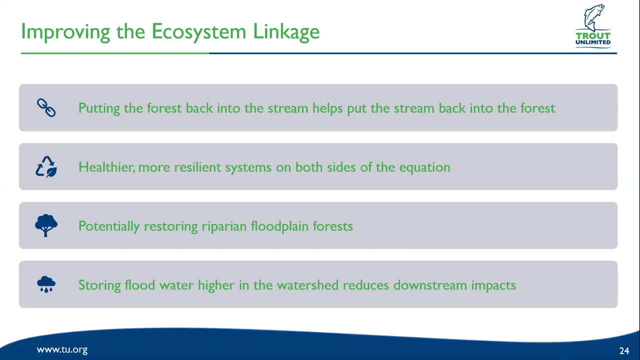 it's just has really high rates of transpiration and can have a big impact on flows, and so this is kind of an interesting example in Hawaii that I wasn't aware of. but it's a neat example and comparison. Great, thank you. When we were talking about- well, I think this is during Aaron's presentation, Jim had another. 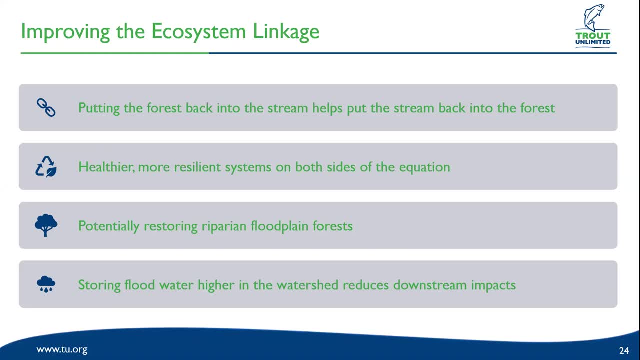 question comment. He says Michigan's current BMP guidance prohibits us from depositing large top trees and logs into streams, even where it would be beneficial. Theoretically we could attempt to get permits for such restoration, but any deposition is now considered a violation In larger navigable streams. we also run up against opposition by some recreationists who prefer 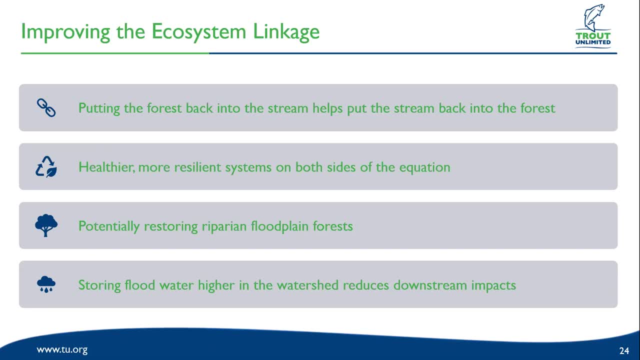 clear runs than few obstacles. And Tim says same story out here. What, Aaron? would you like to respond to that comment? Yeah, I mean definitely what we do. so in terms of forestry BMPs through all the states that we work in, they definitely follow the same regulations. you know, no slash, no. 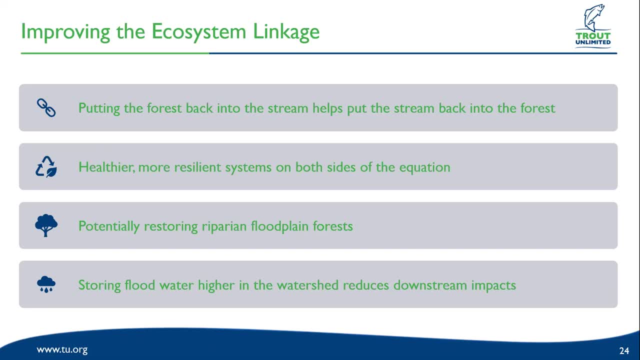 treetops and streams, things like that, But when it is permitted under a as a ecological restoration permit, and especially when it follows certain guidelines, and especially MRCS and others are becoming more aware of this as a practice and are integrating it more and more into forest management plans, even so that private 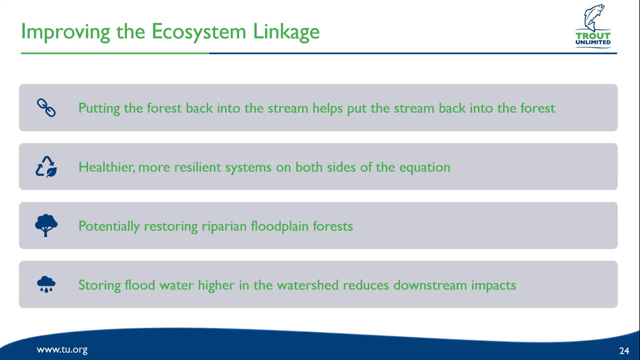 landowners can work with their foresters to actually take these on, And it's been a bit of a slow process. It's definitely been a conversation with a lot of the state agencies to kind of show them the benefits. I think it's really important to do it in small doses and kind of figure out the permitting. 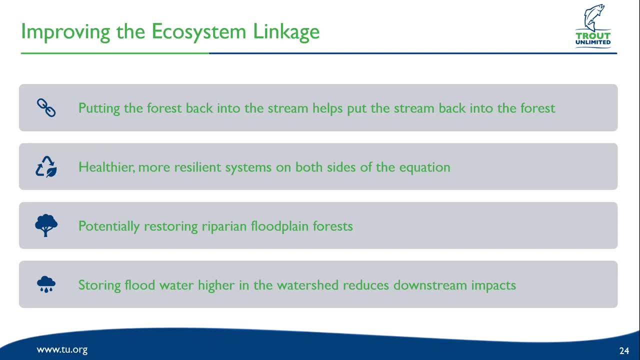 process a little bit slowly, But everybody in New England is really on board with it nowadays And yeah, so it's it's. it is definitely a different permitting process than what I think a lot of forest managers and forest harvest operations have to go through. But that's kind of the next step. 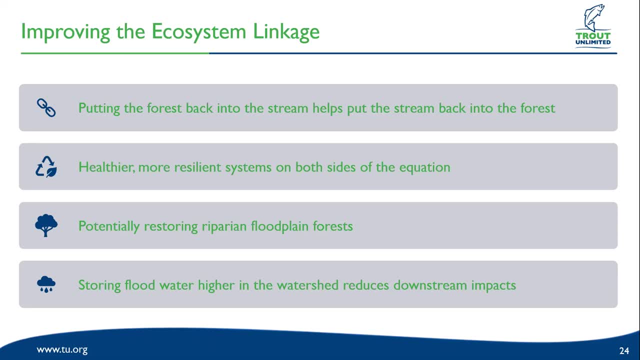 that I've been working with with some of our state agencies. It's kind of how how that can be done together in a responsible way that that bad actors won't be able to take advantage of, while good actors can really, you know, kind of do best works for. 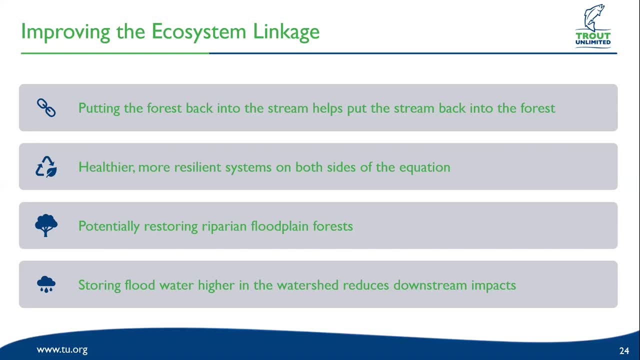 Thank you. Streams. we've actually run into that as well and we've actually gone in and done partial cuts to remove like half a stream width so that there is always a way around some of the larger logs. So I think it's really important to try to get those trees out of the water and get them out of the water. 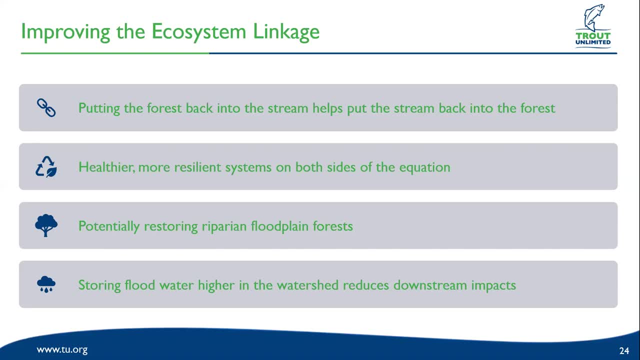 because they can get out of the river as quickly as possible. So I think that's something to look at, But I'm going to turn it over to Karen. Karen Bennett is going to talk about the use of ash to prevent diseases like the beaver and beaver jams, without causing, you know, too much of a risk for paddlers. Got it, thank you. Speaking of how do you get trees into streams, We had a few comments. Karen Bennett said why don't we have some ash and other disease trees to fall in a stream? And we also had a question about reintroducing beavers, as there are in the west. Maria replied that many people in northeast will comment that beavers are reintroducing themselves. I don't know if you have a comment on more natural beavers or not. 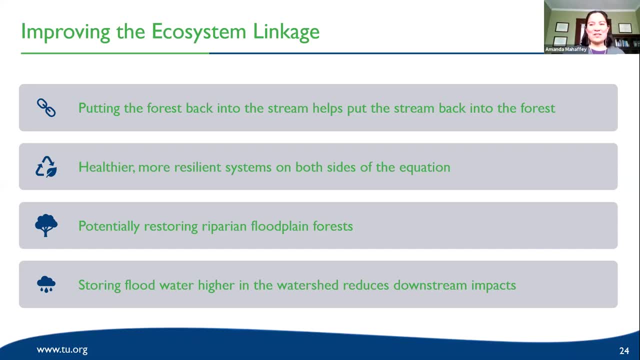 ways or opportunities to get trees into streams. Yeah, I mean, that's why we definitely leave standing dead. We know that they're gonna make their way in there eventually and we don't take all of the ash. We know that. or in hemlock woolly, adelgid areas, we don't take all of the hemlocks. We're still kind of. 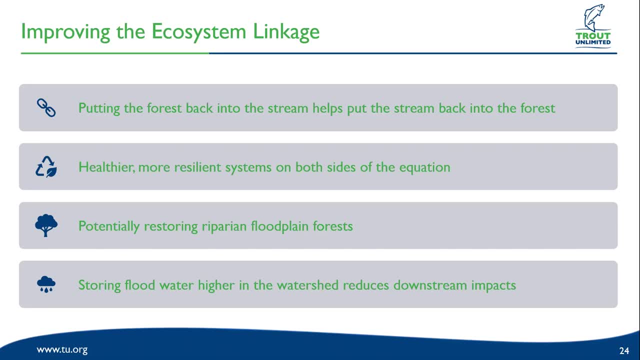 maintaining those. generally, you know, not more than four or five trees in an area of an installation, so that, yes, there is still a lot left over that will naturally recruit over time, depending on how quickly disease moves through what kind of rates of decay around the base. And so, yeah, in terms of the beaver, yeah, 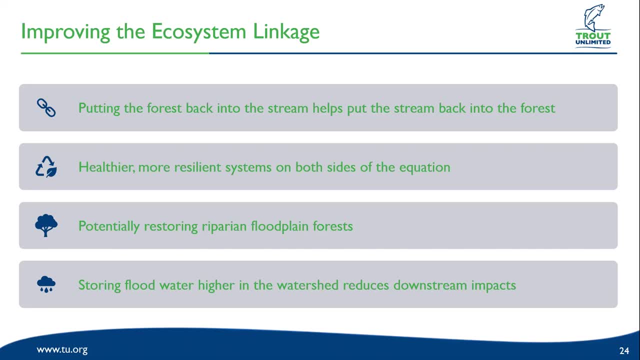 there are still a lot of folks who don't want to see beaver in a lot of areas. I think they do a lot of wonderful things for a landscape and they're actually quite expensive. I've been to a couple of at the special- actually a lot of people who have been looking into doing beaver dam analogs. 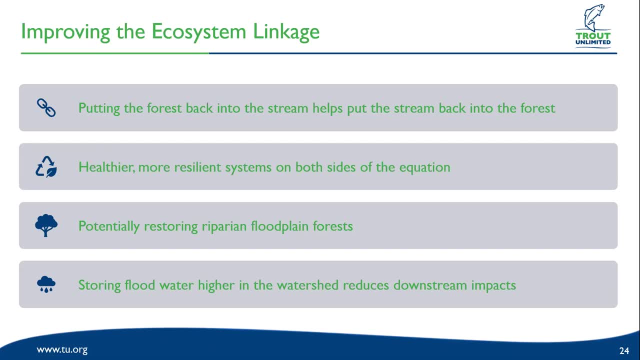 which is basically human-built beaver dams where beavers do not exist, and that's had some really good results too for areas where people don't necessarily want the beaver but they still want the ecological restoration. Cool, thank you. We're getting some really awesome questions into the group chat. 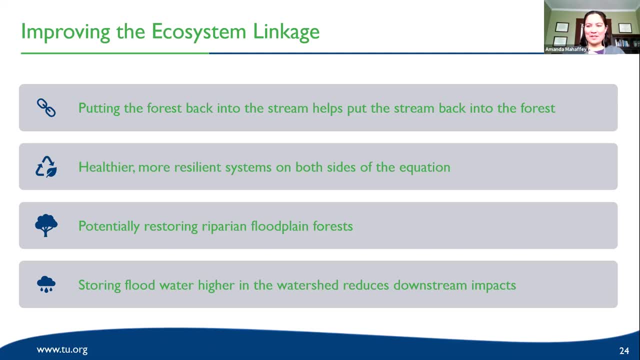 For a quick timeout. I think our speakers are able to stay on a few minutes after the top of the hour, so I think we'll keep questions going as long as they come. But in the meantime I will go back and I will pause just before the top of the hour to make sure we get good information out. We 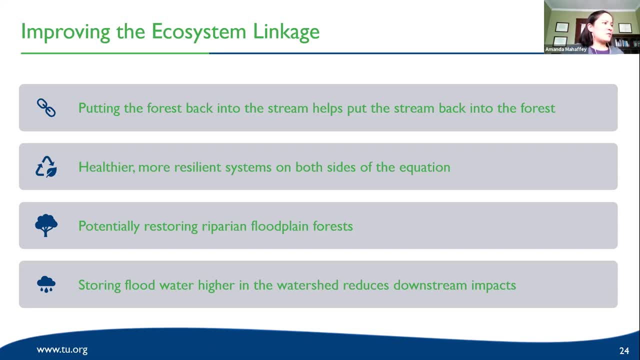 had another question that came into the chat box from Adam, who asked: would maintaining higher volumes of woody debris during average and low flow conditions mitigate the impact of wood moving during peak elements, ie by slowing down the water flow And reducing the volume of wood moving downstream during those and the damage 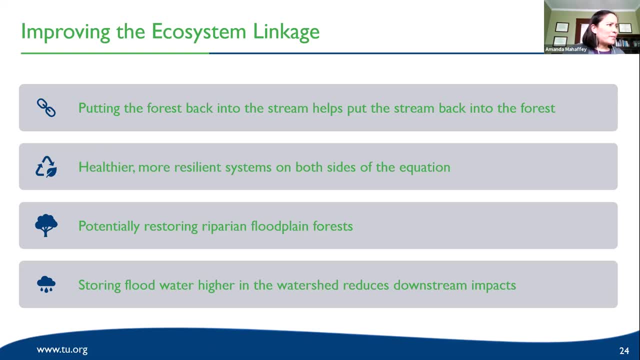 to infrastructure By slowing flow and reducing the volume of wood moving downstream during those and the damage to infrastructure. perhaps the peak flows overwhelm any slowing effect of the larger wood and thus have the opposite effect, ie more wood damaging infrastructure. Maybe there's a short. 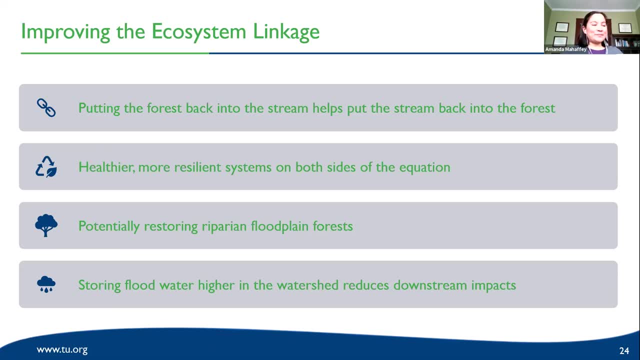 versus long-term trade-off here as well. Yeah, it's hard, I feel like to quantify that at this point. I mean we've seen enough wood moving off the landscape in systems that don't have any wood naturally occurring, or much natural wood occurring in streams and still damaging. 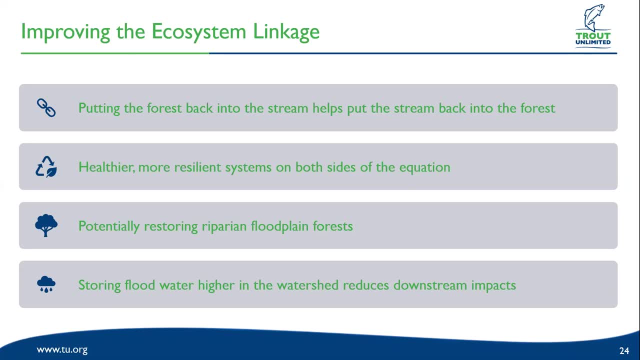 infrastructure during those high storm events that we don't typically, I mean. so we, we do take a lot of measures to make sure that there's going to be a lot of conflict And you know there's no consensus on whether a peak would be as little mobile wood. 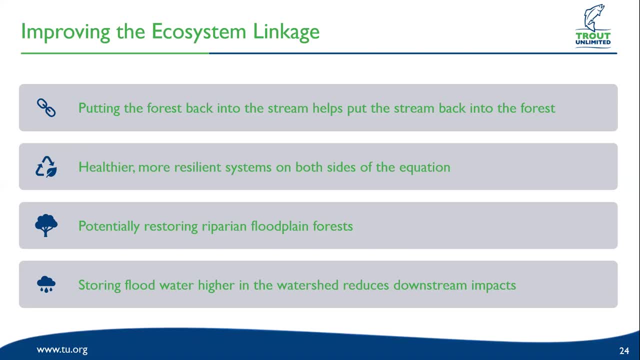 during most flow events. So we have ways of securing things by natural means without bringing cabling or other things into the mix. Perhaps this peak flows of the one the slowing effect? Yeah, I mean, there's already plenty of wood-damaging infrastructure in terms of short to very Slow activity for some of the 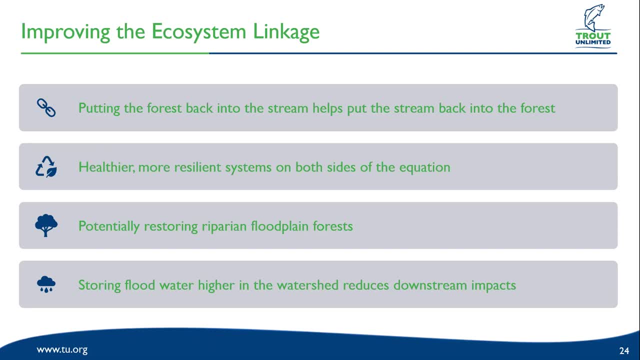 infrastructure Okay versus long-term trade-offs. And I mean, I kind of hate to say, but there are a lot of towns that replacing infrastructure has gotten to be expensive enough that they're actually waiting for it to fail so that they can replace it more easily. 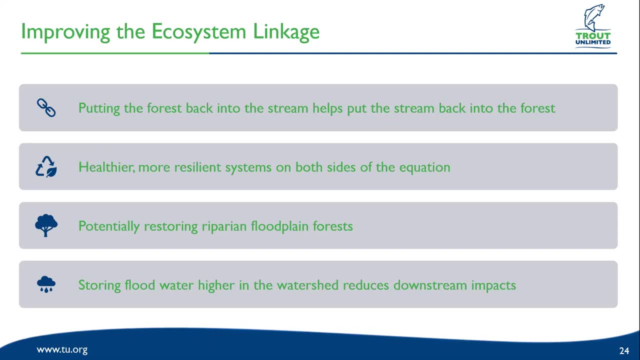 without having to pay for the removal because the stream just did it for them. And I mean I certainly don't want to advocate that as a route that anybody should be taking, because there's a lot more damage done during those emergency replacements than good most of the time. 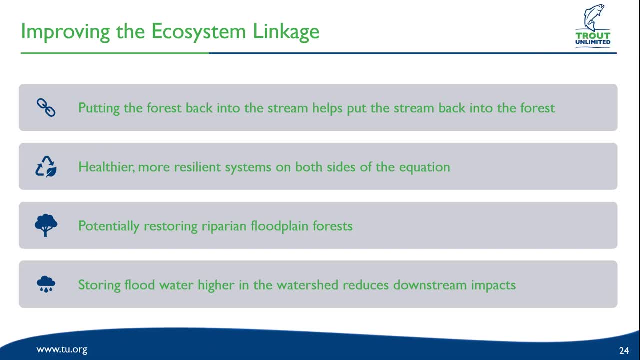 So, yeah, it's definitely a short versus long-term trade-off, But I feel like anything that can mitigate these large storm events high up in the watershed, where there is a lot less infrastructure to be at risk, is gonna be a benefit for most communities. 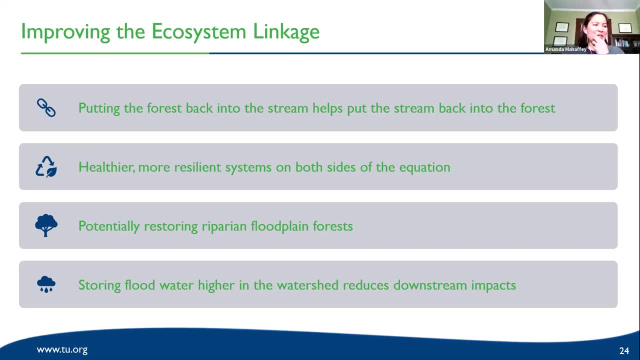 So I think that's a good question. Thank you, I'll see if we can get Jonathan to answer a question. Nicole just asked: do you have any downstream water quality data that shows improvement in turbidity or other water quality parameters? post-ecological restoration effort. 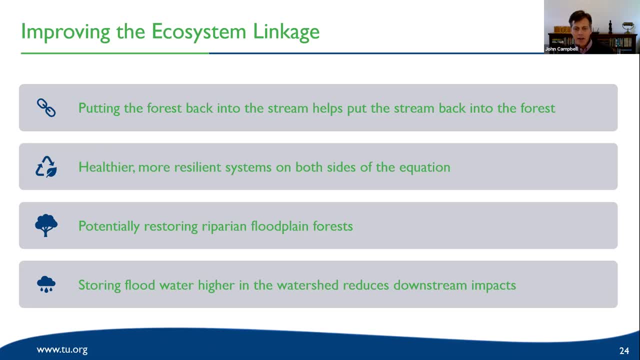 Yeah, so I'm a little confused by the question. So that is like, well downstream, So yes, so I think that's more of a question for Aaron. right, And in terms of the restoration with woody debris At Hover Brook, we don't really do restoration so much. 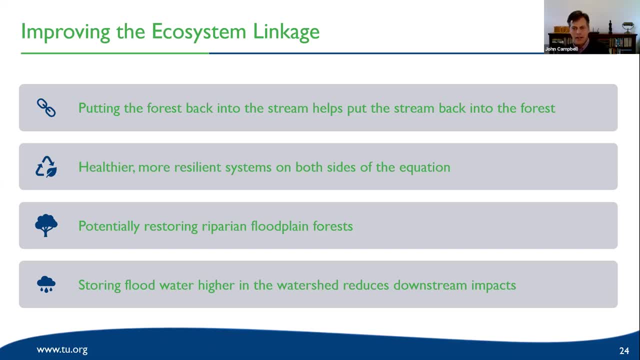 We've had these cutting experiments, and all those are done at the watershed scale, And so we monitor the chemistry and have an understanding of the impact, But we don't do much in terms of water quality improvement. So maybe that's a better question for Aaron. 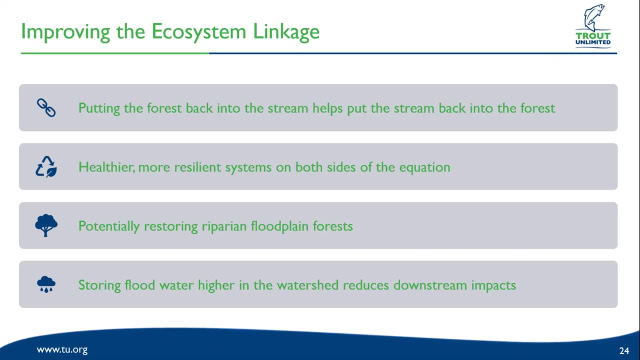 Okay, thank you. So there has been a few studies that are still kind of in their preliminary stages. as far as I know, There was one that we were working specifically with the University of New Hampshire Water Center and a few of their grad students who were doing nitrogen monitoring. 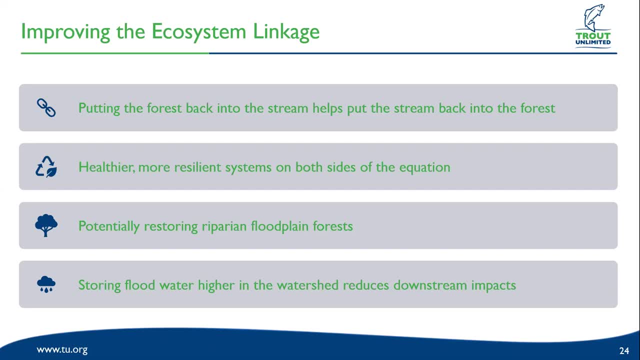 at several of our locations. Initial results have shown that it certainly does help in nitrogen reduction kind of at a much larger reach scale within the river. But I don't think anything has been published out of that yet. so Okay, good question. 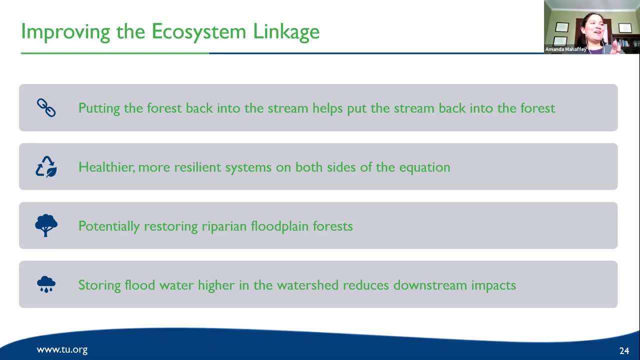 Thank you. I'm gonna take a quick time out here and there are so many questions. we're gonna have to keep going, but I know that a lot of people might need to jump off at this time, So we will keep going, but please join me in a virtual thank you to our presenters. 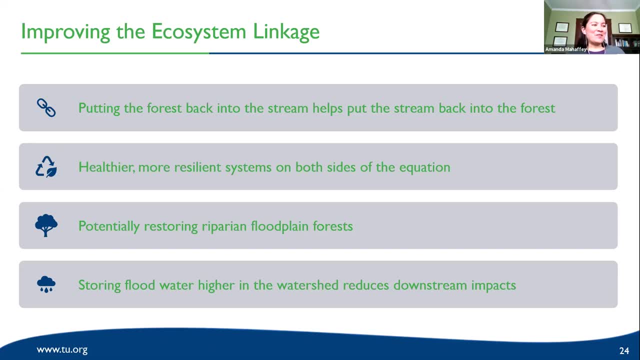 This has been a really, really active and engaging webinar, So thank you. I also wanna point out that I did put in the chat box a link to the SAF CFE certificate, So it's the Certificate of Credit Assignment, And if you didn't get the link, 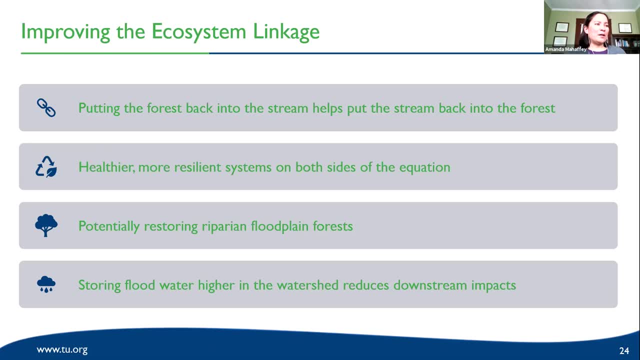 I can email it to you later. Just let me know if you need it And I will be reporting the participant list to SAF for anybody who is seeking credit. But if you need the certificate for your own records, then we'll have that available. 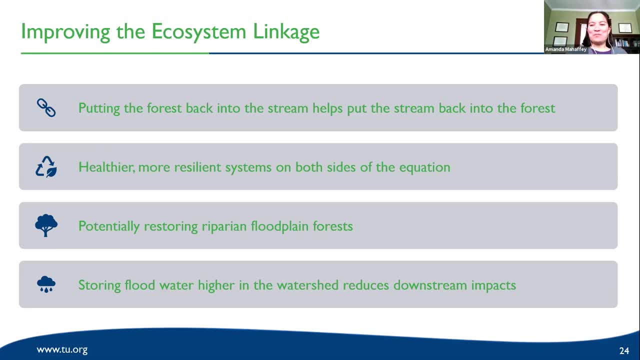 With that, we're gonna dive back into questions. Thanks again to Erin and John for sticking with us, because we've got some really good ones in here. Oh great, Where to begin? Where to begin? Nancy Patch had a really good question. 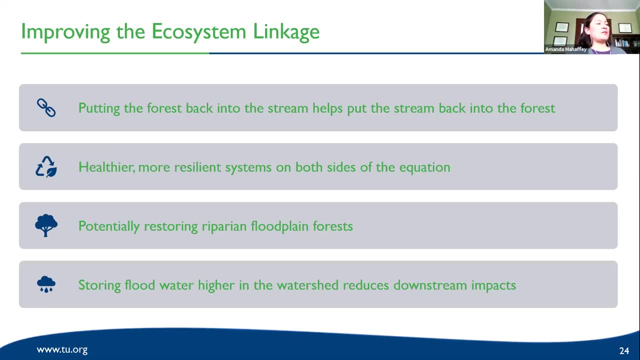 She says. I'm wondering about the management of our wood road infrastructure outside of our carried area: historical roadwork, ditches and drains disrupting the natural sheeting and hydrologic flow, resulting in concentrated flow. Should we be designing our roads differently? Maybe more outlets and angled roads? 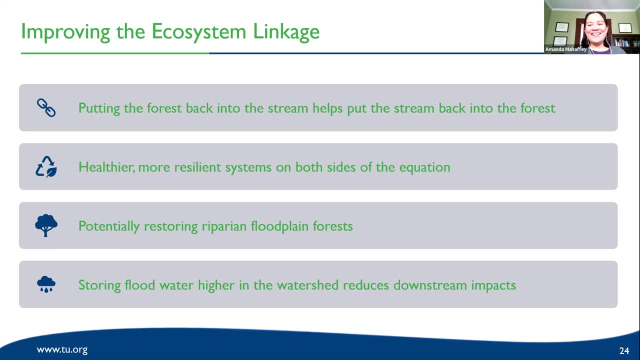 like the old dozer roads. Either of you could take that. I mean that's a little tricky an engineer, but you know, I think there is probably, you know, more care that can be taken and thought put into some of these road networks and how they're constructed, especially in some 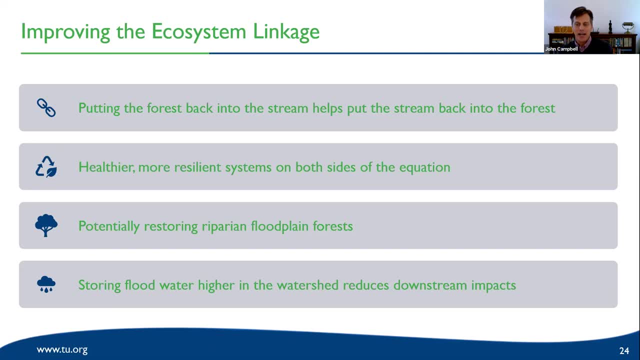 of these forested areas. BMPs do cover a lot of that and so, but certainly I think there's probably more that could be done there. I mean, I've been working with a few towns just in terms of their. you know, Vermont has a lot of dirt roads- Western Mass, New Hampshire. 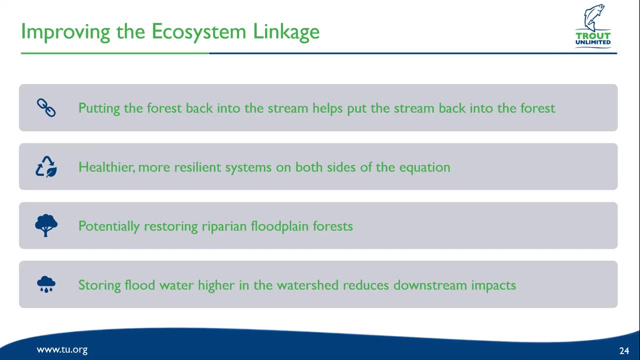 all those areas and you know they run into a lot of the same problems in terms of you know what works in terms of flow and drainage and what is just which roads are continually washing into the stream, no matter what they do. So that's definitely an ongoing. 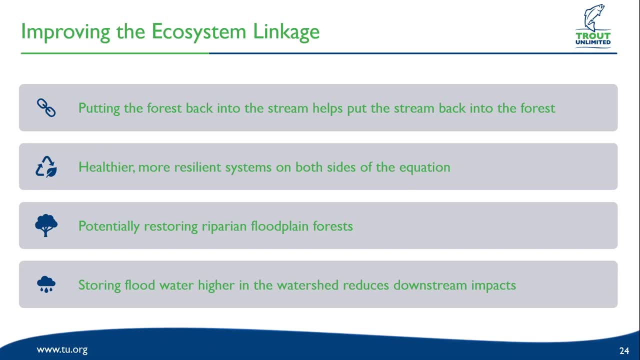 conversation- an ongoing project- that people are still trying to find solutions to Not being nearly as well-versed in logging roads and their construction. I can't answer as much to that one, though Sounds like a good research project, which might tie us to our next question. 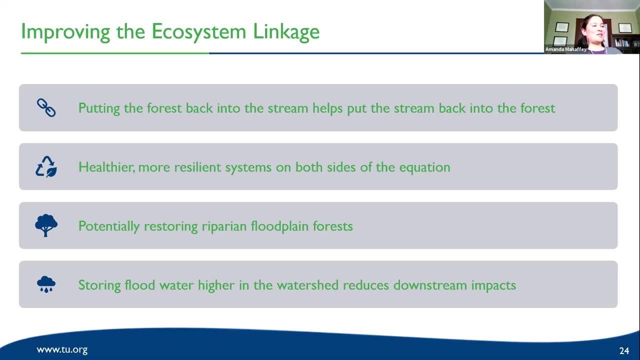 Stephen has asked: has Copperbrook considered implementing Trout Unlimited wood installations on a subset of their study area and then analyze the hydrologic effects to that stream? A good collaborative opportunity here, possibly. Yeah, that's a great suggestion. So I'm not sure if I can answer that question, but I think it's a good question. So I'm not sure if I can answer that question, But I think it's a good question. I think it's a good question, So I'm not sure if I can answer that question. So I'm not sure if I can answer that question. 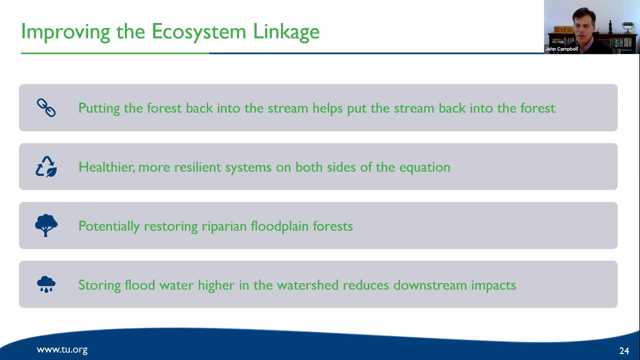 At Hubbard Brook there's been a long history of doing wood additions and removals and debris, dam additions and removals And the Hubbard Brook streams- a lot of them are first and second order streams and the focus of that was not so much on fish as it was on more biogeochemistry. 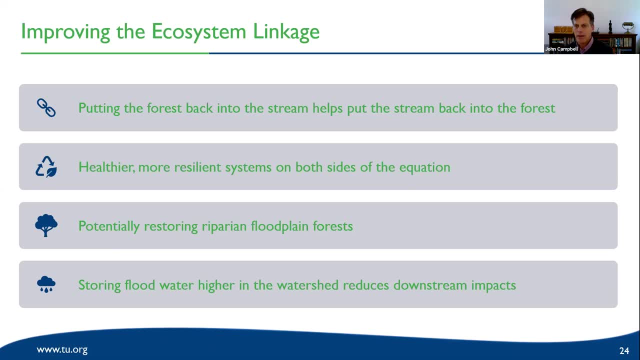 Most recently, Bill Keaton at the University of Vermont has a proposal that's funded to do some of this work and look at the role of woody debris in streams, and he's trying to figure out methods. It's still in kind of the design phase now, but this is something we're going to be actively. 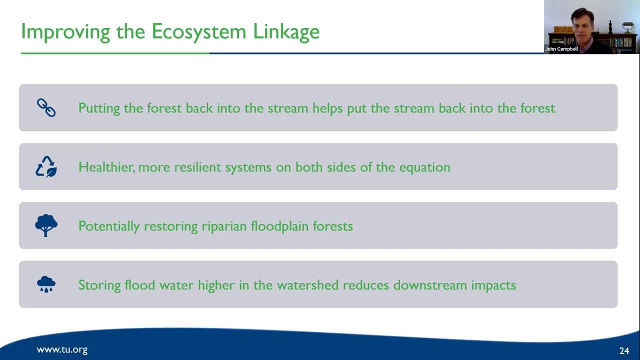 working on, People who fish at Hubbard Brook are often go away very disappointed because there aren't a lot of fish, just because it's kind of difficult terrain in these real low order first and second order streams And so we don't have a lot of fish, but there are some brook trout and a few other fish. 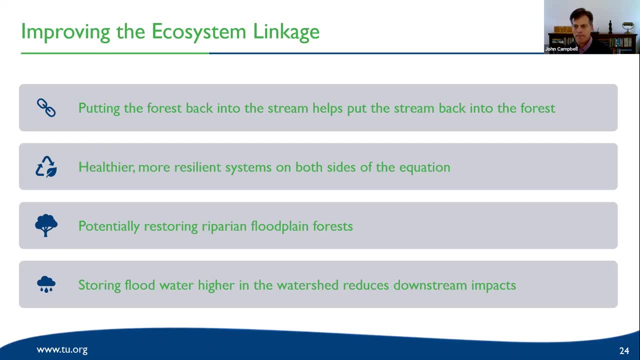 species. Cool Erin, did you want to add to that or are you good for now? Yeah, no, I mean I'm happy to collaborate with nearly anyone who has land to kind of implement this work and especially who has the capacity to really dig deeper into some. 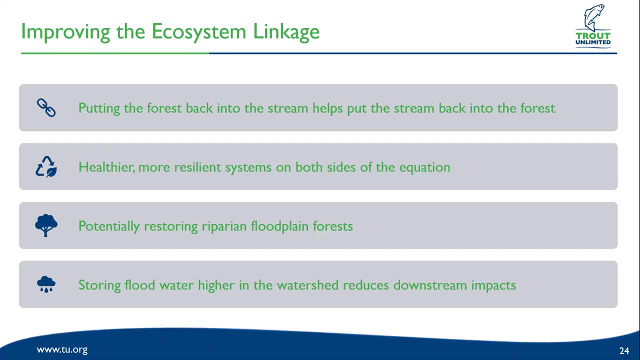 of the effects that this is having on the landscape scale In terms of benefits to fisheries and particularly to recreational fishers. We do get some complaints, that you know the messy nature of this work, especially early on, puts off a lot of people. but you know, over a series of years, several studies, 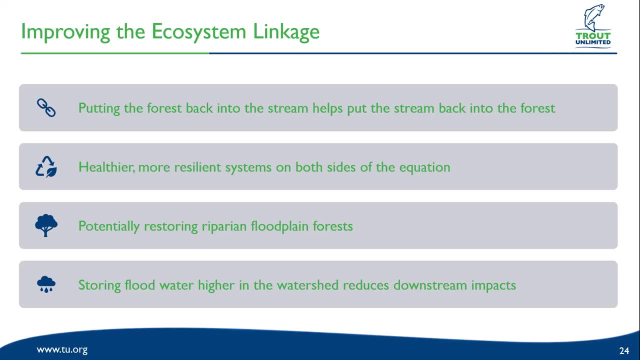 by Jud Kratzer up in Northern Vermont who does similar work to this. he's found, you know, 300% increases in the size and abundance of brook trout in the streams where you know these restoration techniques have been put in. 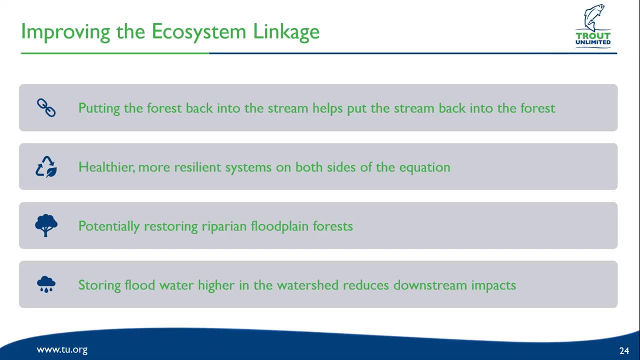 So it definitely helps on the longer run, but you just have to be a better fisherman to do it All right. Speaking of fish, someone asked how did trout get past the log jams? They are actually a lot more, you know, permeable than they look. 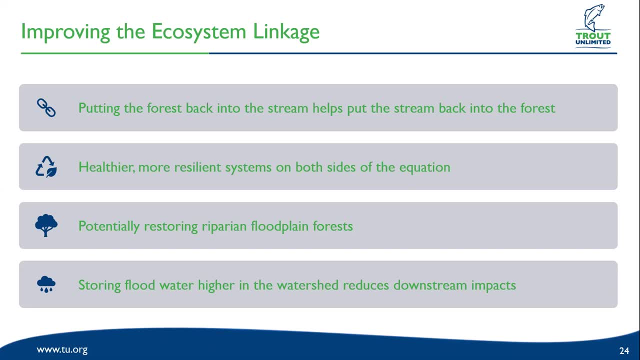 It's not easy for a human to get through, but when you are, you know, a fish that is just a few inches long, it's a lot easier. for sure, Yeah, Got it. Thank you. Jim had a question. He says I would be interested if we might have success simply girdling a few bigger. 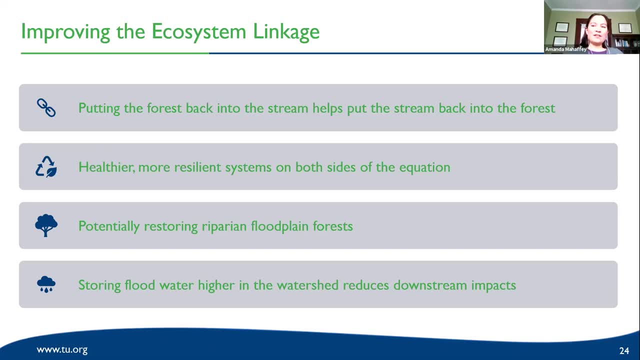 lower quality trees within the riparian zone, Yep. So I actually work with a few land trusts and when we were first piloting some of this work and how we could integrate it into private landowners' forestry management plans through the land trust, that was one of the first steps that they actually started taking before. 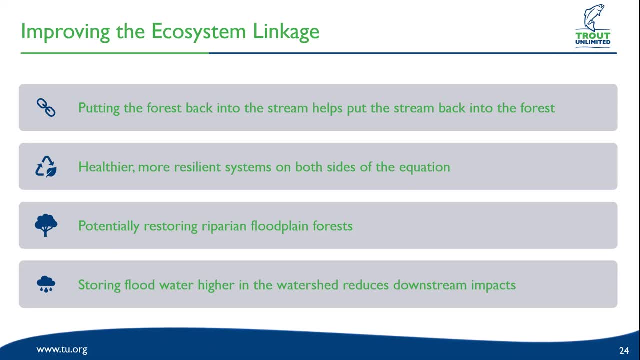 the cutting in stream would happen. Yeah, So one of the things that they really kind of took off was, you know, girdling trees, kind of setting up that you know standing dead tree to eventually, you know A become. 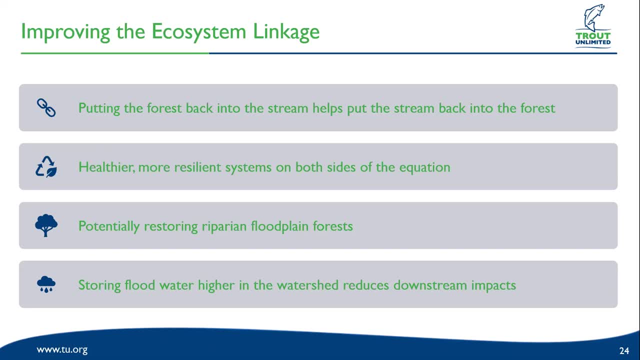 good habitat for a range of things, and then to eventually fall into the stream as well. It's definitely a longer range goal, but forestry management plans usually are, And so I'm certainly supportive of that. It's also a consideration, though, too right. 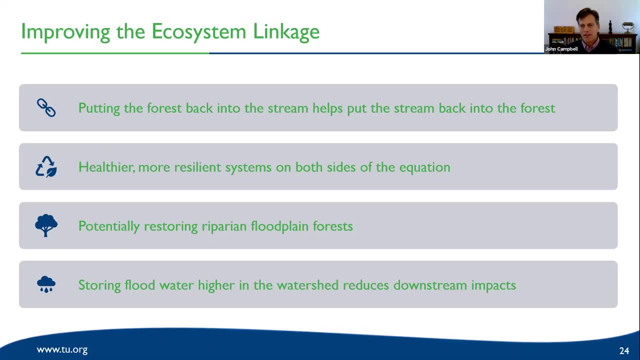 I mean, that's something you don't have any control over. when it will fall Right? So you don't want to be doing that in areas where there are people regularly. Yeah, Yeah, Definitely, Sure, Yeah, I'll try to get a couple more questions in. 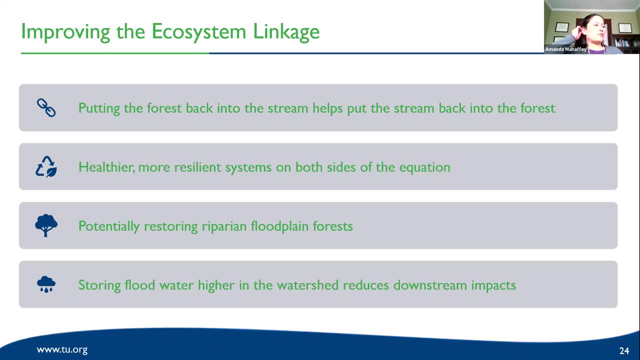 Tim asks: in addition to cutting experiments, are you using prescribed fire for forest and watershed health? I don't, because I am not a forest or a fire person. That's okay. I don't know if it's done anything that way, Okay. 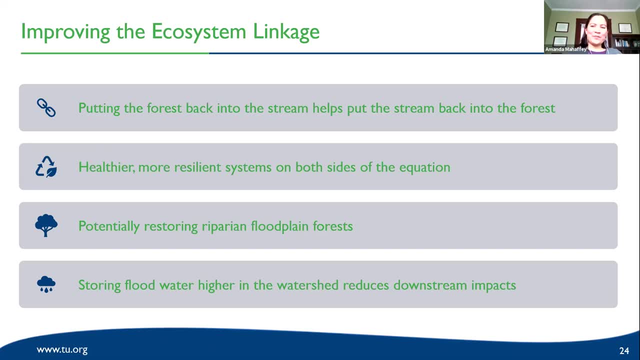 So we haven't done much with fire. It's a hard sell in the northeast And so, even though we do have occasional fires, it hasn't been a high research priority. I've personally tried to get things funded to look at fire and have failed miserably. 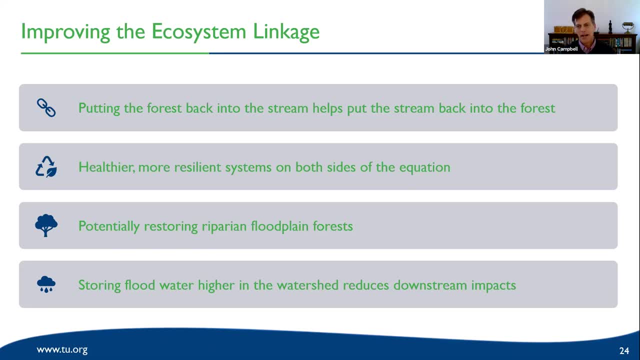 And so it hasn't become a high research priority. It's not to say it won't be in the future, but right now it's really hard to get that kind of work funded. Yeah, Thanks for that. Yeah, Awesome, Thank you. 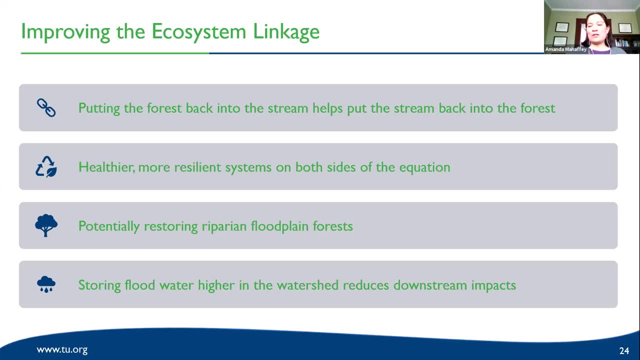 We have another question. We have a question from the North Atlantic Fire Science Exchange And maybe we should chat more offline, John, It would be fun to look at questions like that. But yeah, prescribed fire is not as common here as it is out west, but it does still. 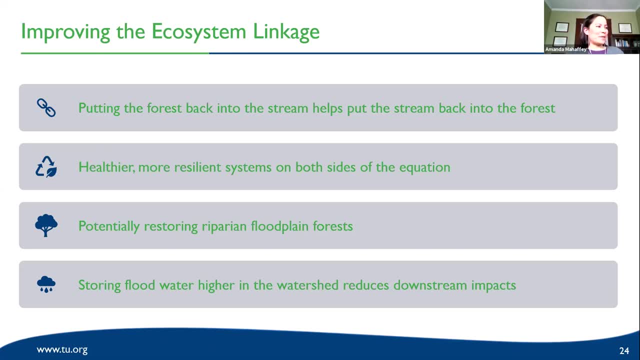 happen And so maybe there's some possibilities there. Last question Dominique asks. in 2006,, a major rain on snow event at Mount Rainier created tremendous flooding in the park. Streams in the park now have enough sediments from glacier melt that water level and road. 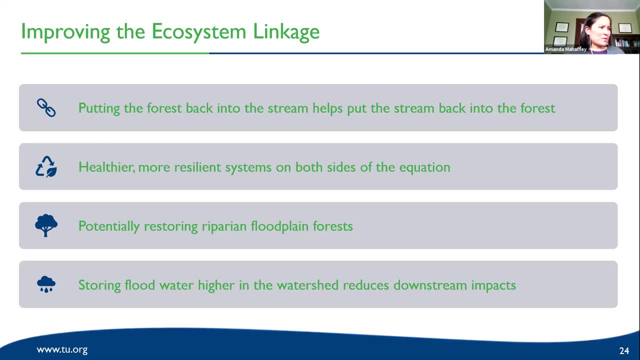 level are even thus mega flooding always possible? The park was closed for six months then, but staff and engineers restored the entire road system at the exact same place. Any advice about more long-term vision for restoration after the next major flood event? I think this sort of thing happens a lot. 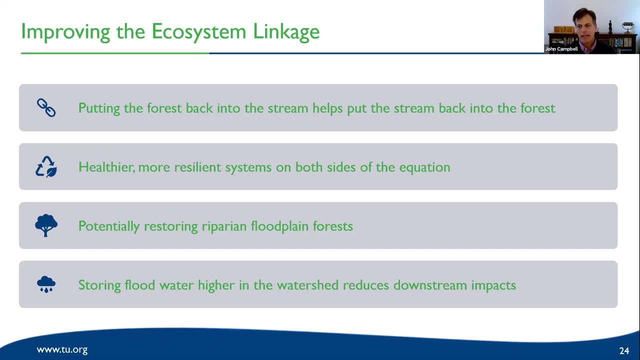 I think it happened on the White Mountain National Forest after Hurricane Irene, where many of the culverts they replaced they replaced with culverts of the same size because that's what they were budgeted for, And so I have been trying to make this case. 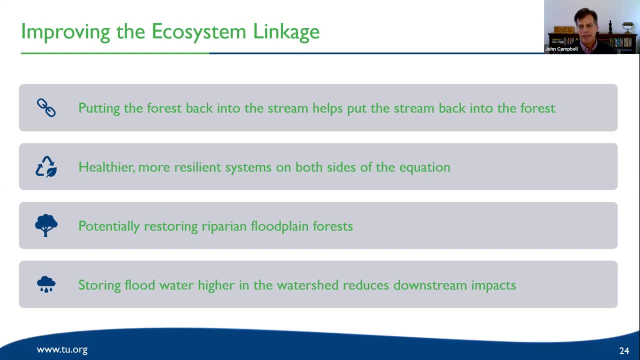 And I think a lot of people are realizing how important it is to really think about the future, as I said in my presentation, when kind of designing these things, It's not what's happening now, It's what could happen over the next 50 or 100 years. 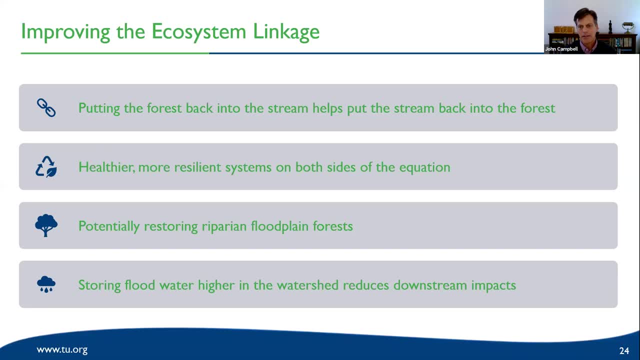 And it's so important when infrastructure is designed to last for a long period. Yeah, And I mean the whole stream and road flooding all the time. Yeah, It's a regular occurrence, I think throughout New England. I mean, a lot of the roads were always built in floodplains because it was the easy flat.